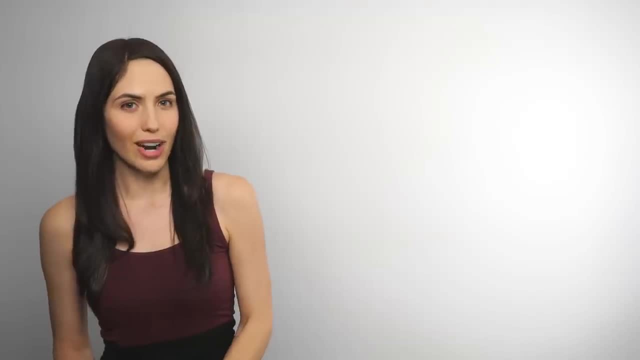 Hi guys, I'm Nancy and I'm going to show you how to solve a right triangle, which I know sounds pretty vague. Like what does that mean exactly? It just means find all the missing sides and angles, And it's not that bad. Let me show you how to do it. 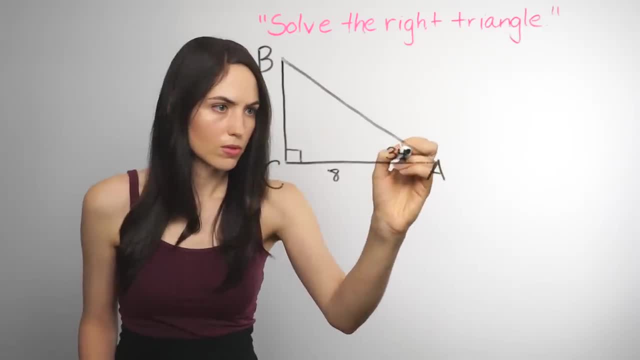 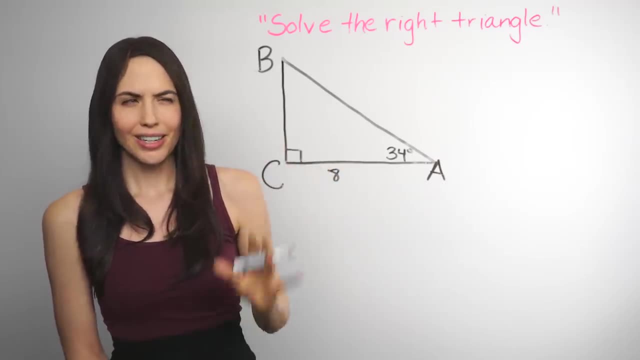 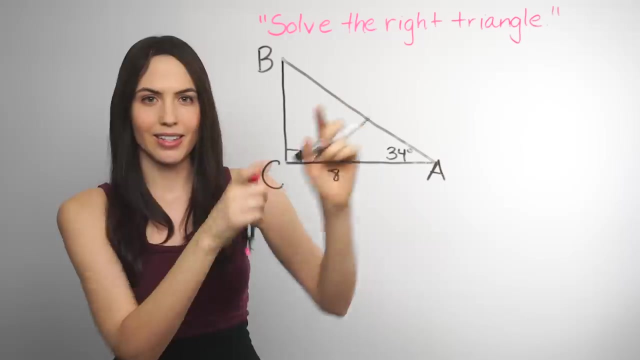 Alright, say you have a right triangle and you're supposed to solve that right triangle. I know it's a little unclear. like I said, it's a little vague as to what that means. It just means find any missing sides or angles that are not already labeled on your right. 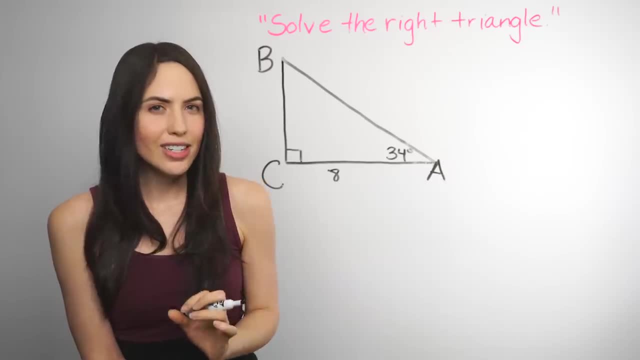 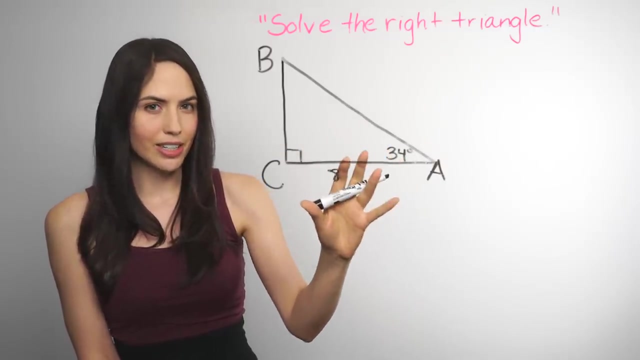 triangle And I'm going to show you how to do that. But first, just in case you were wondering if this is some kind of special right triangle like 30-60-90 or 45-45-90, I'm showing you this one on purpose, because I know that 34 degrees is suspiciously similar. 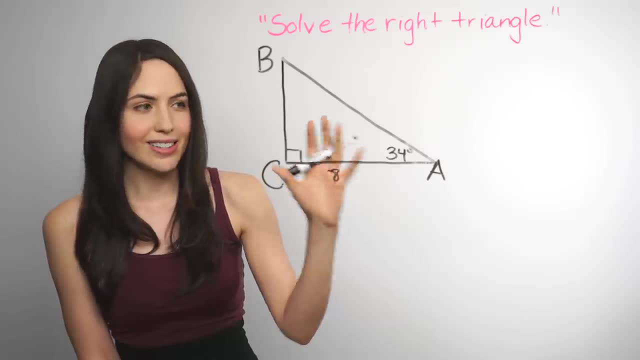 to 30 degrees. But unless you have exactly 30 degrees as an angle, or 60 degrees or 45 degrees, it's not a special right triangle, Not so special. So we can't use those. What can we do? Well, 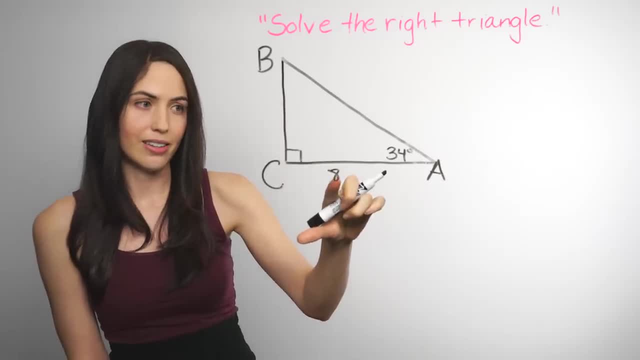 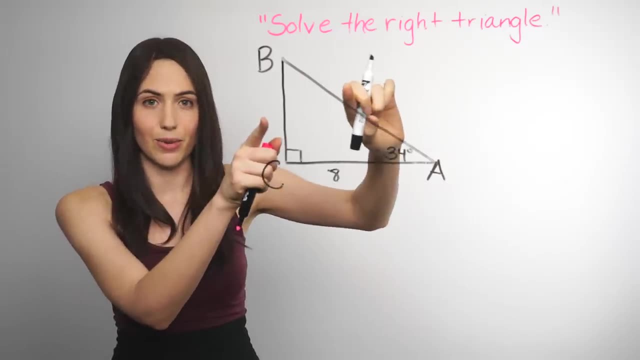 if you have a right triangle and you know at least one side and an angle that's not the right angle, you can use a trig function to find the sides that you don't know, And the first thing to do is to label those sides that you don't know, And then you're going. 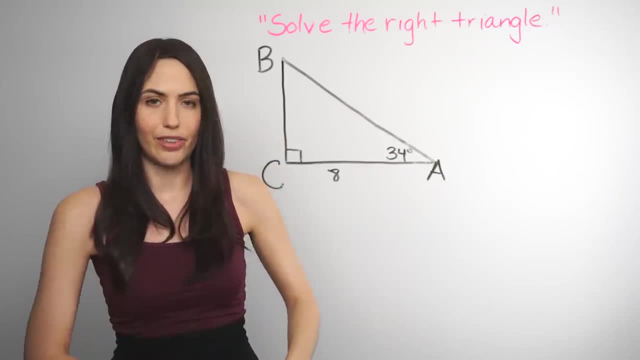 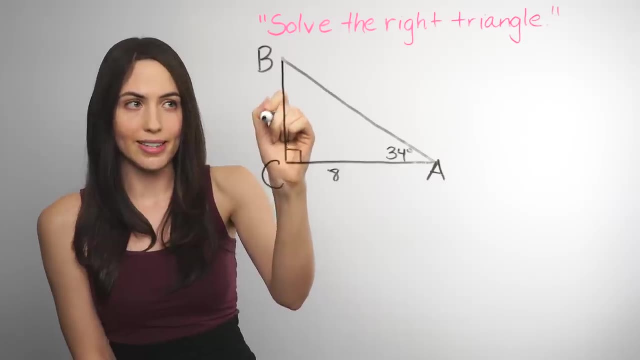 to give them names that you're looking for, that you don't know. Give them names. They deserve that much, the dignity of having a name. And you can use whatever letters or variables you want. I'm going to use lowercase a and lowercase c And I'm just using those. 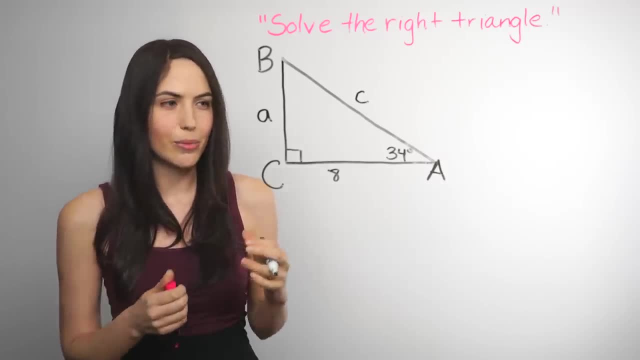 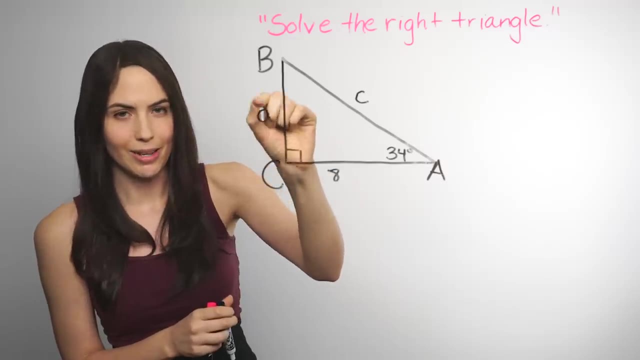 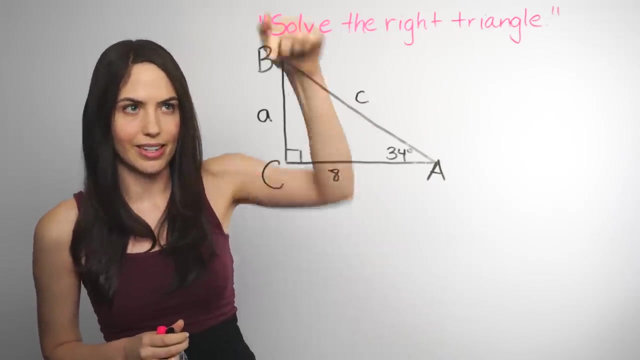 because there's this convention, this standard. you might see where, for the big A, the angle, capital A, the side that's directly across from it, a lot of times is labeled little a, lowercase a. The side directly across from capital C is little c And the side directly across from 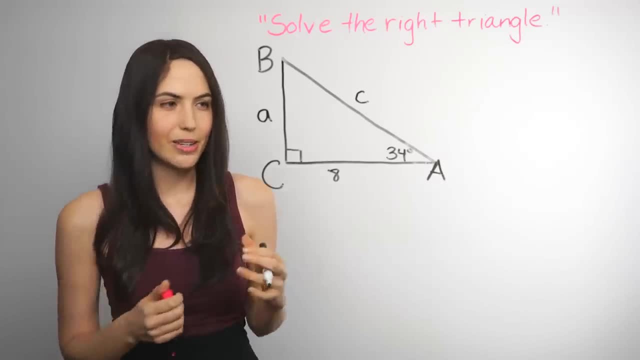 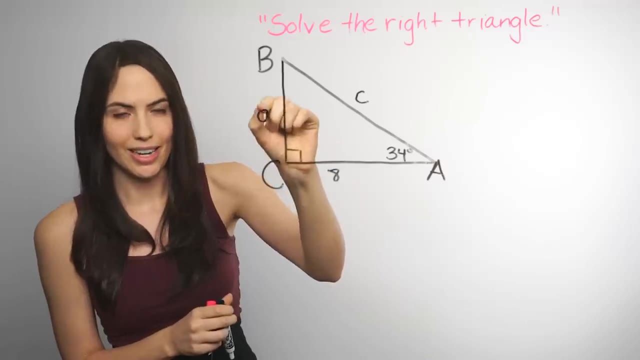 because there's this convention, this standard you might see where for the big A, the angle capital A, the side that's directly across from it a lot of times is labeled little a, lowercase a. 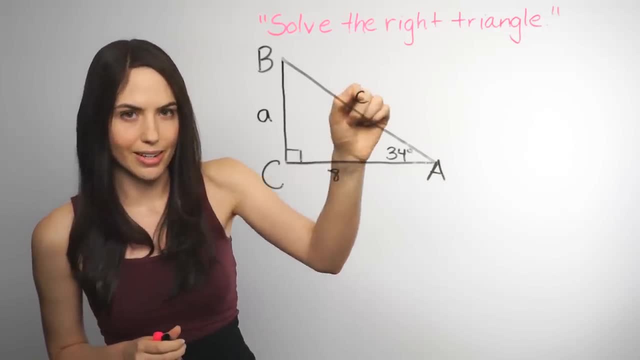 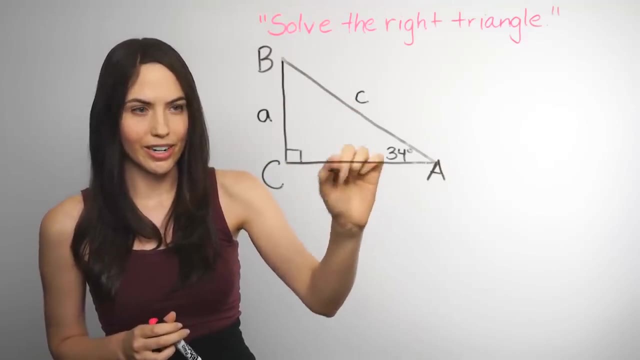 The side directly across from capital C is little c. And the side directly across from capital B angle is lowercase b. But we don't need that because we already know what that 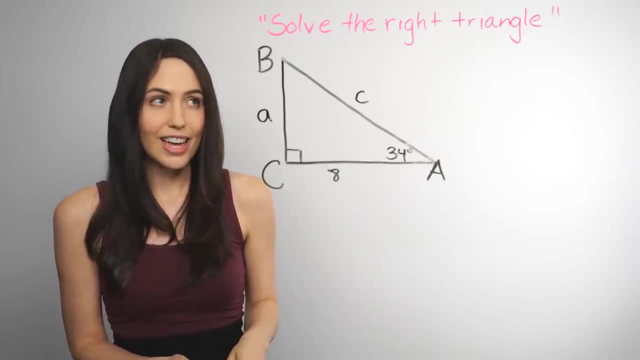 is, 8. So I said that you could use a trig function to find each of these sides, but how do you know which trig function, sine, cosine, tangent, to pick? Good question. 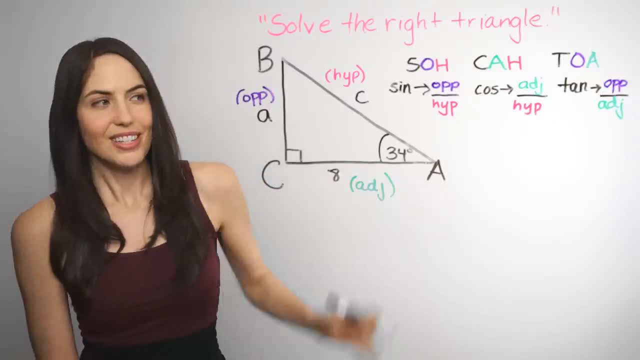 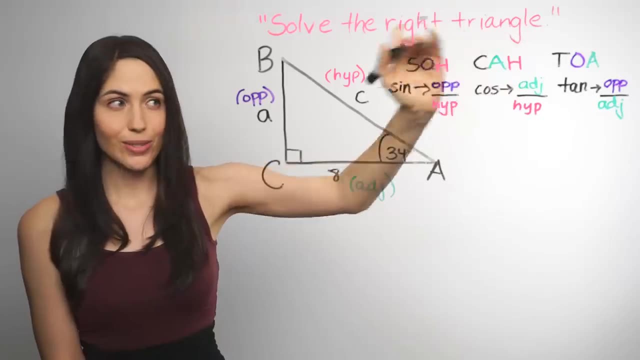 All right. So these are three of the main trig functions, sine, cosine, and tangent. This is a memory trick, SOHCAHTOA. It's a mnemonic device meant to help you remember 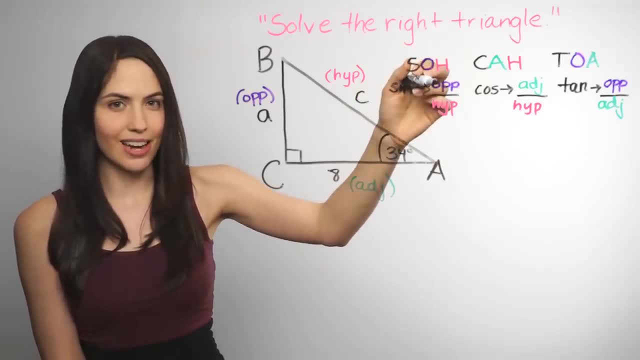 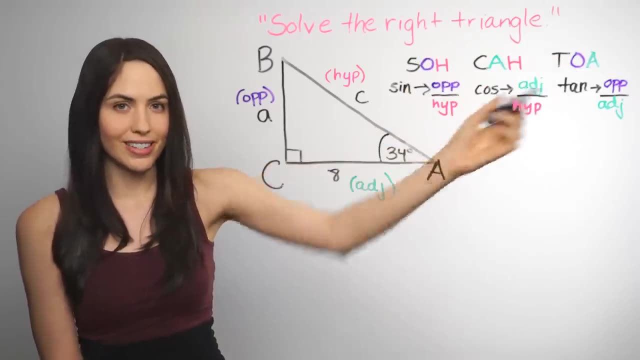 that sine of an angle is equal to the opposite side over the hypotenuse. Cosine of an angle is adjacent over hypotenuse. Tangent of an angle is opposite over adjacent. What are 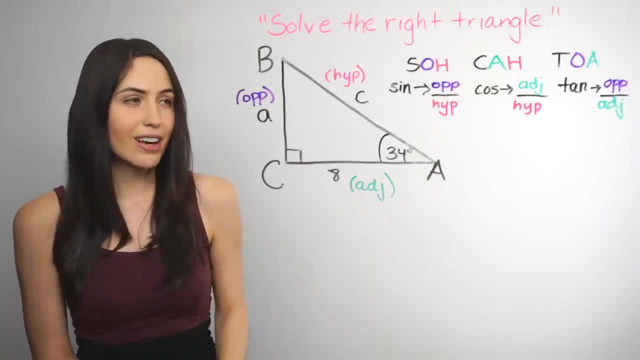 these opposite, adjacent, hypotenuse things I'm talking about? I'm going to give you a little bit of a look at this. So if you don't know, you can go to my other trig video and 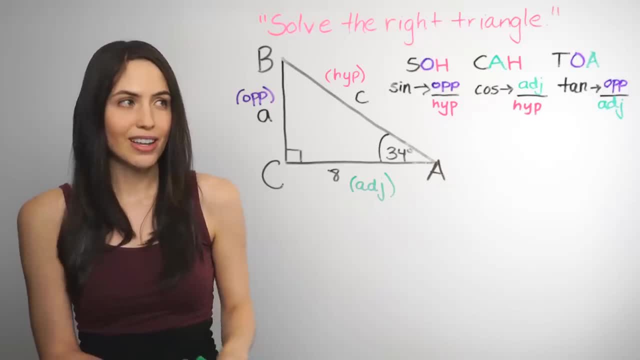 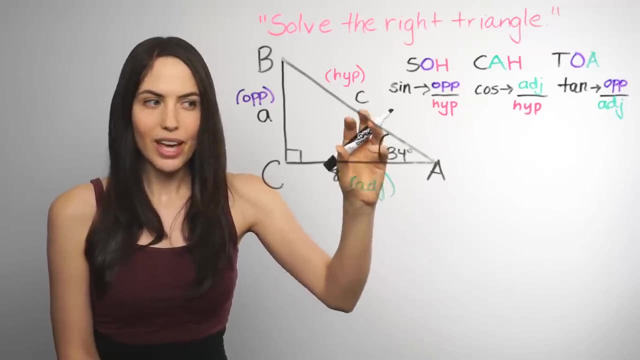 jump to that. I do a whole introduction and explanation of that. But basically it depends what angle you're focused on, what angle you're looking from. We have this 34 degree angle 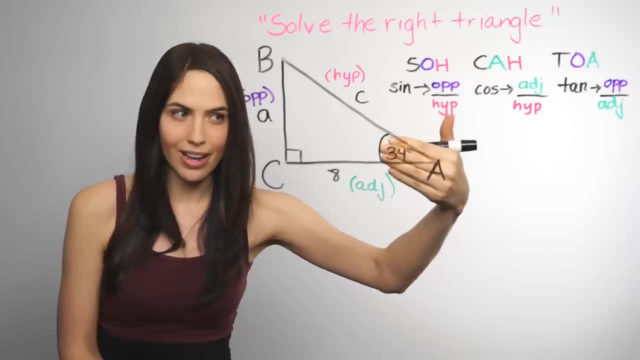 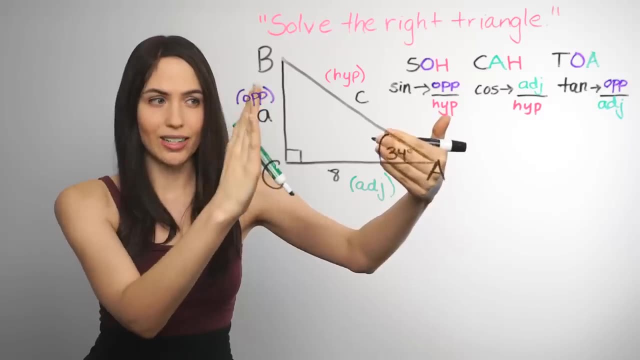 in our triangle. From the point of view of that angle looking out, from its perspective looking out, this is the opposite side because it's directly opposite that angle, directly across. 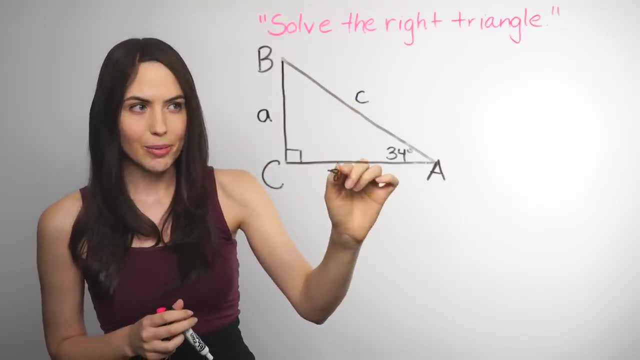 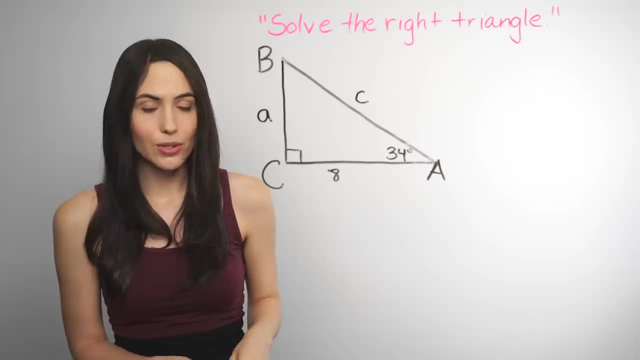 capital B angle is lowercase b. But we don't need that because we already know what that is: 8.. So I said that you could use a trig function to find each of these sides, but how do you know which trig function, sine cosine tangent, to pick? Good question. 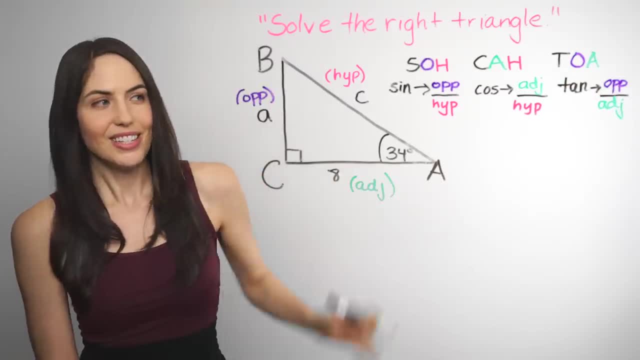 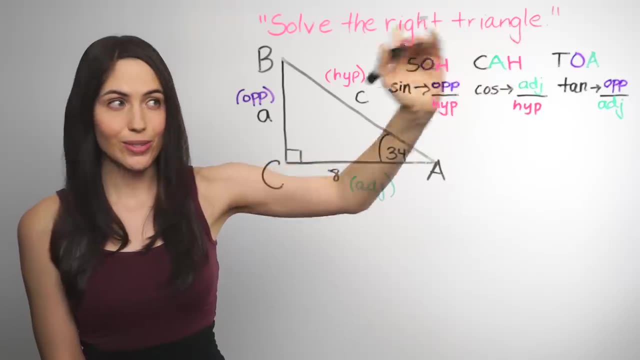 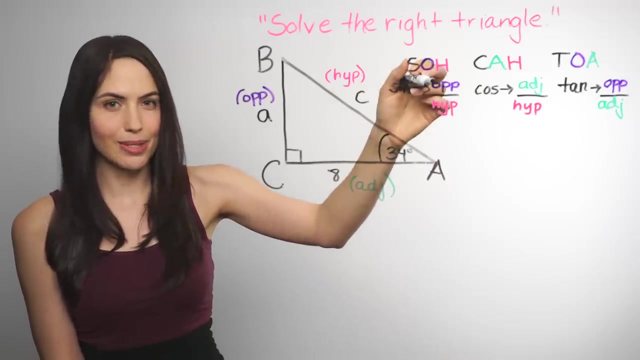 All right. So these are three of the main trig functions: sine, cosine and tangent. This is a memory trick, SOHCAHTOA. It's a mnemonic device meant to help you remember that sine of an angle is equal to the opposite side over the hypotenuse Cosine of an angle. 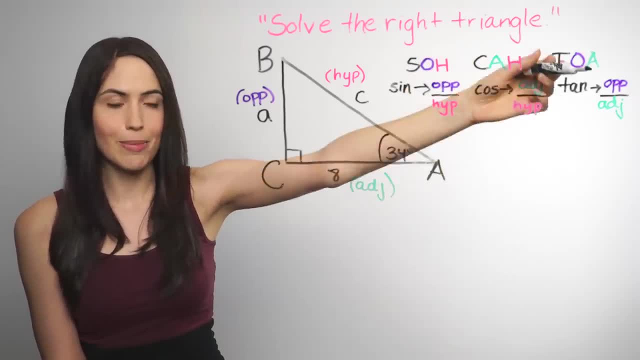 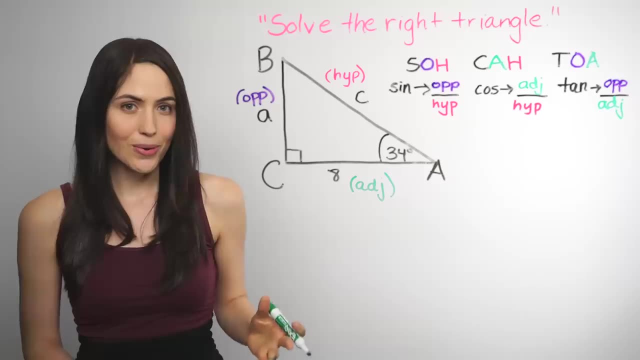 is adjacent over hypotenuse. Tangent of an angle is opposite over adjacent. What are these opposite, adjacent hypotenuse things I'm talking about? If you don't know, you can go to my other trig video and jump to that. I do a whole. 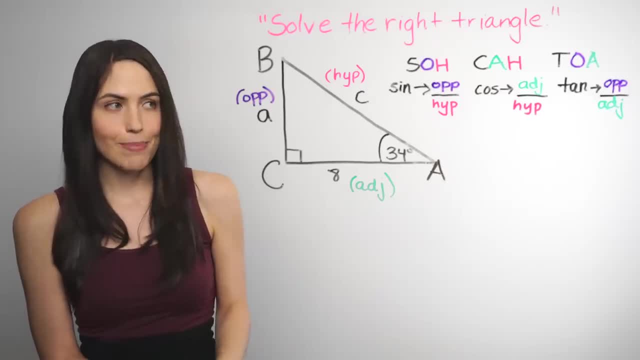 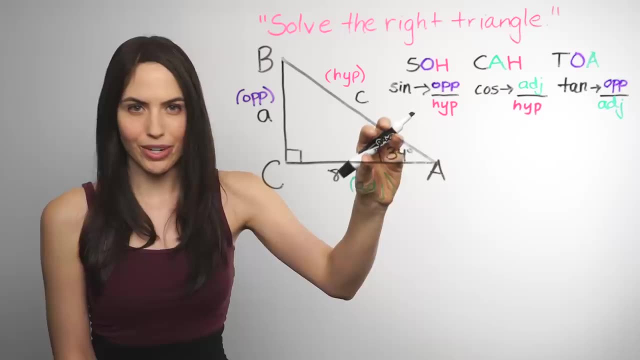 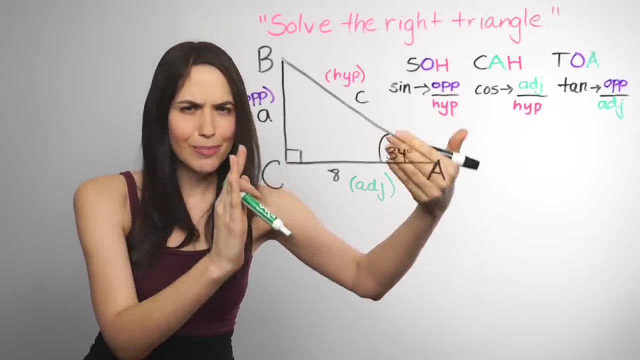 introduction and explanation of that. But basically it depends what angle you're focused on, what angle you're looking from. We have this 34-degree angle in our triangle. From the point of view of that angle, looking out, from its perspective, looking out, this is: 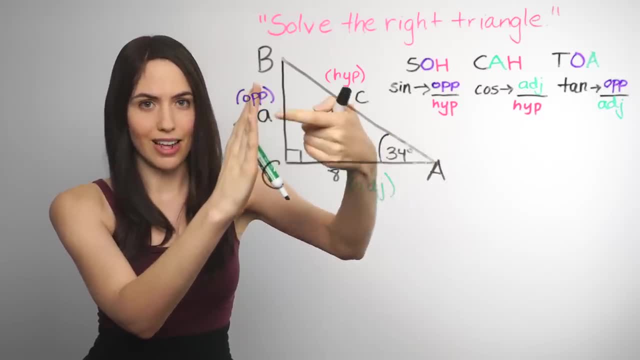 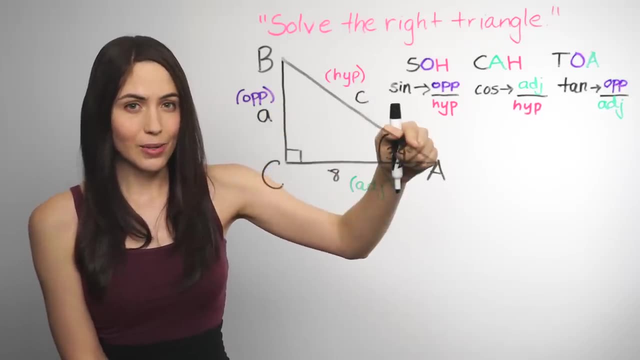 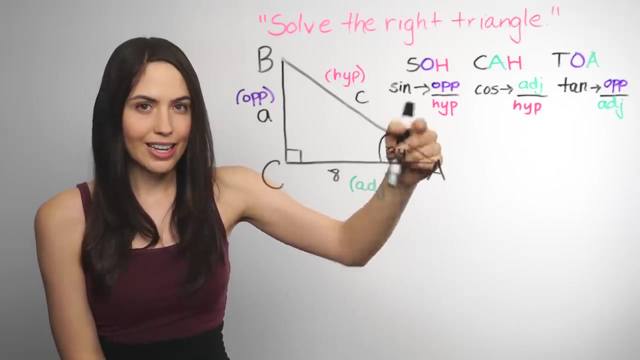 the opposite side because it's directly opposite that angle, directly across. Okay, Opposite side. The longest side is always the hypotenuse, the one that's straight across from the right angle, the 90-degree angle. It's always the hypotenuse And then the other. 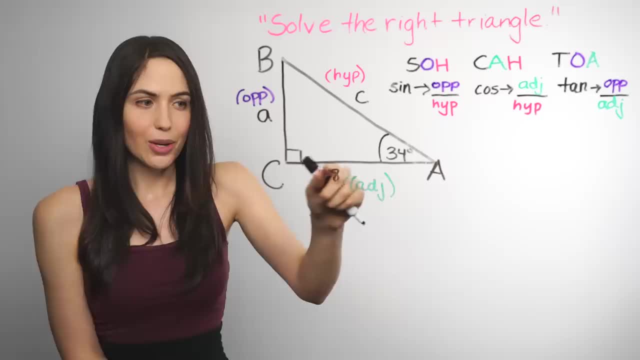 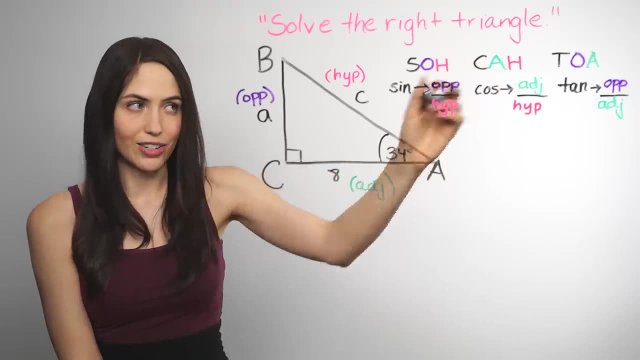 side that's next to our angle but is not opposite and is not the longest side. is the adjacent side ADJ or A in our trig? So how do you know which of those three to pick? Well, say that we want to find out which of these three to pick? Well, say that we want to find out. 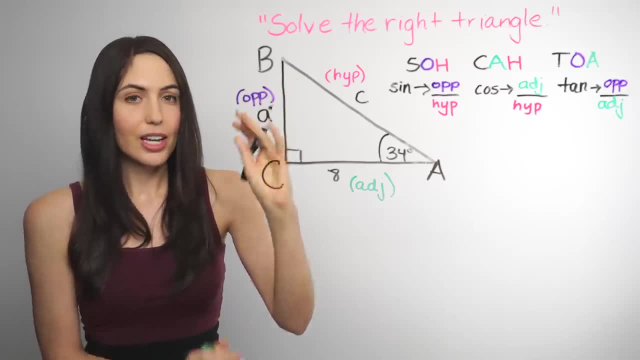 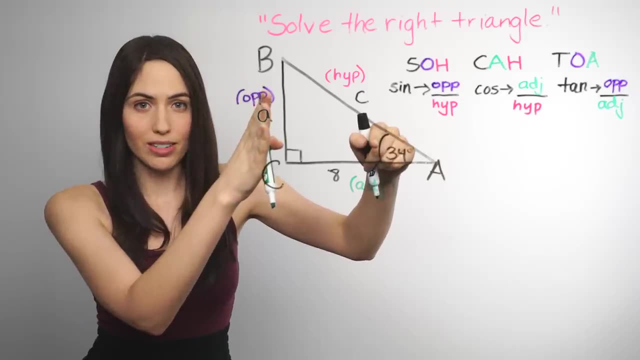 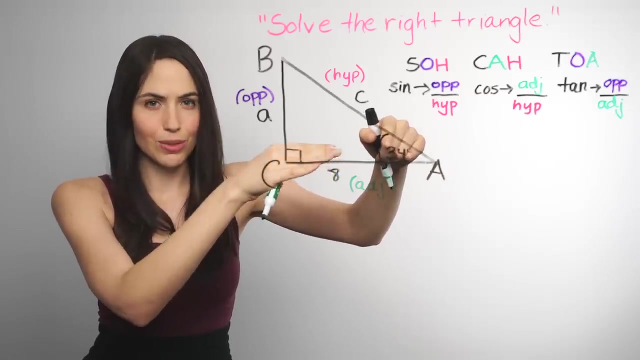 this side, Suggest that we pick one of the other three. Listen again And on a paper knife we're gonna initialize our activists to find this side, solve for A. Here's the rule of thumb: Pick the one of these three, pick the one that includes both the side that. 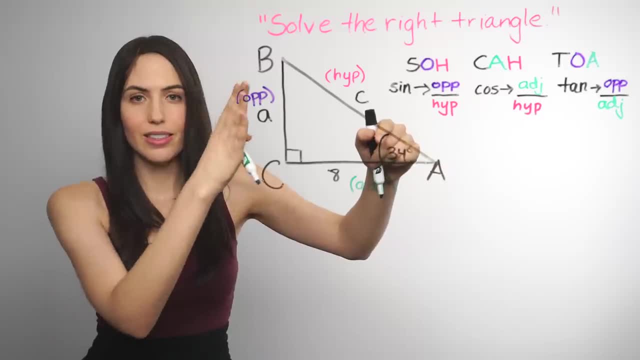 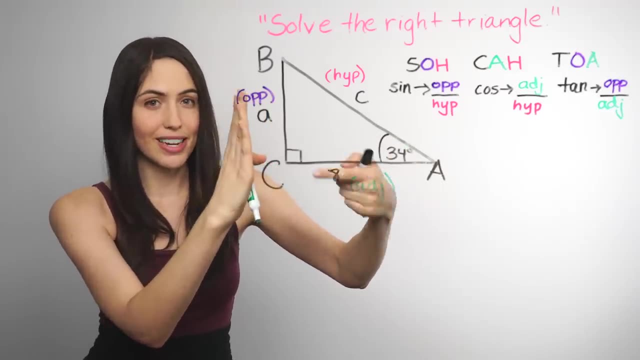 you want, that you're looking for, that you don't know, and the side that you know, something that you do know, the number for the value. We want one that includes the opposite and the adjacent, because we're looking for A and. 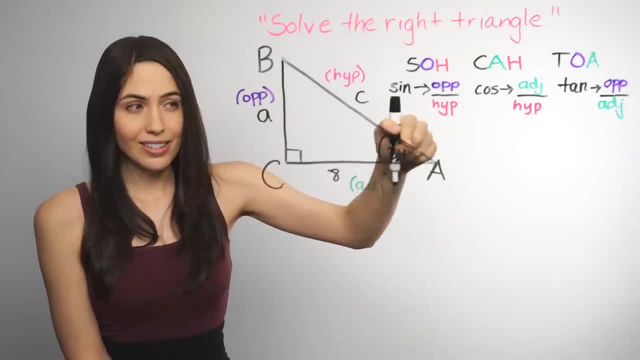 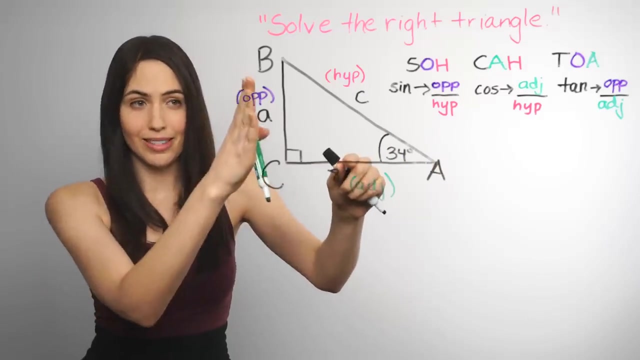 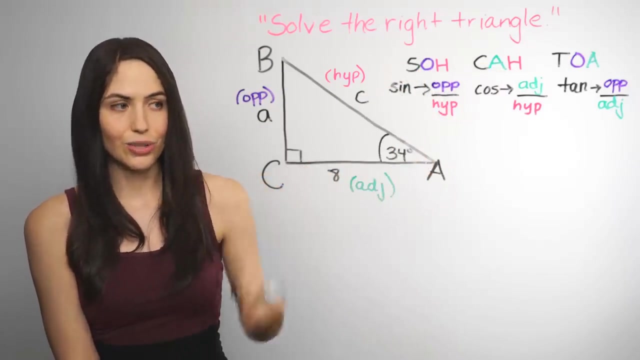 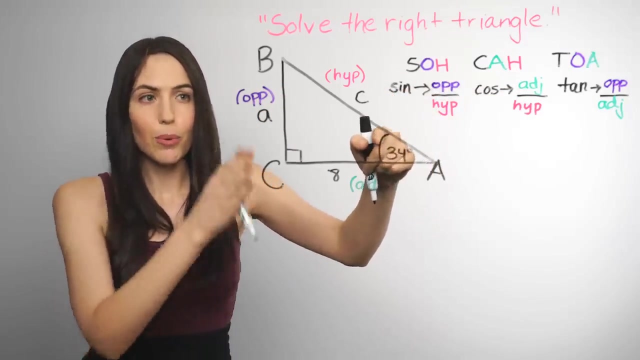 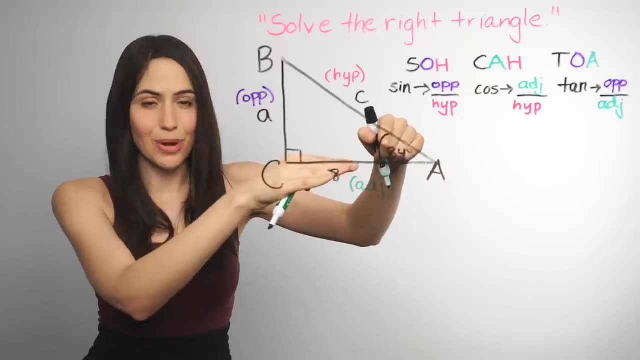 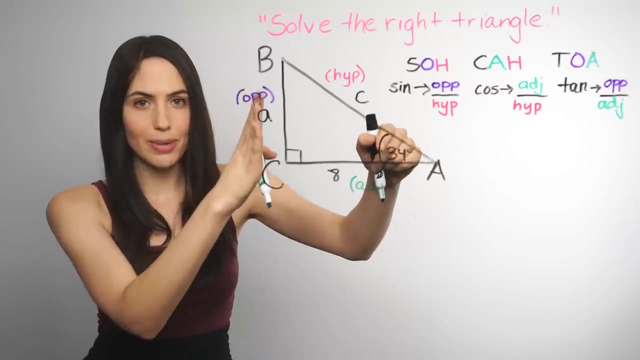 Opposite side. The longest side is always the hypotenuse, the one that's straight across from the right angle, the 90 degree angle. It's always the hypotenuse. And then the other side that's next to our angle, but is not opposite and is not the longest side, is the adjacent side, ADJ or A in our trig. So how do you know which of those three to pick? Well say that we want to find this side, solve for A. Here's the rule of thumb. Pick the one of these three. Pick the one that includes both the side that you want, that you're looking for, that you don't know, and the side that you know, something that you do know the number for, the value. So we want one that includes the opposite and the adjacent because we're looking for A and we have 8. 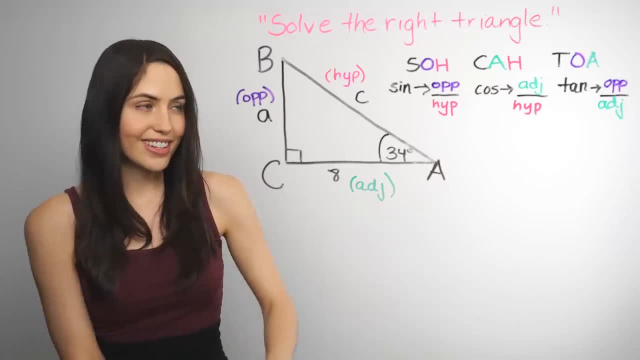 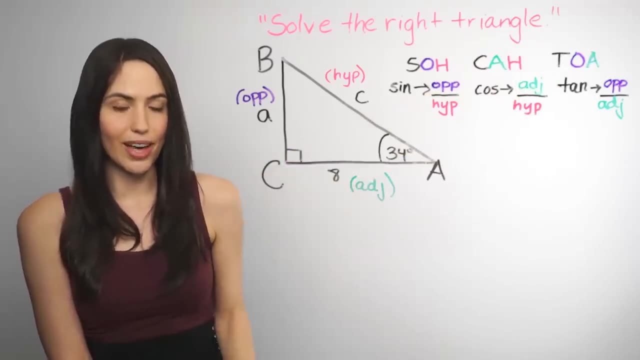 Opposite and adjacent. O and A, you may have already guessed, is tangent trig function. Tan is opposite over adjacent. O, A. The TOA in SOH CAH TOA. So all we have to do now is write a little equation. 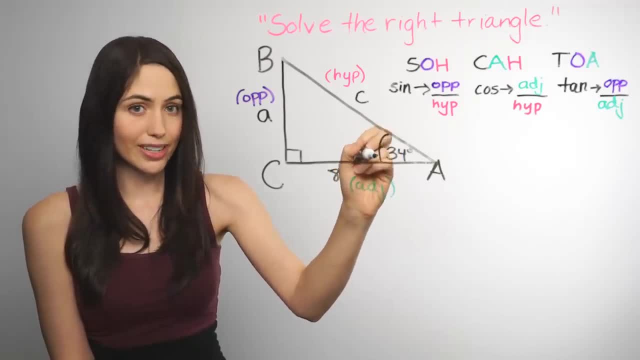 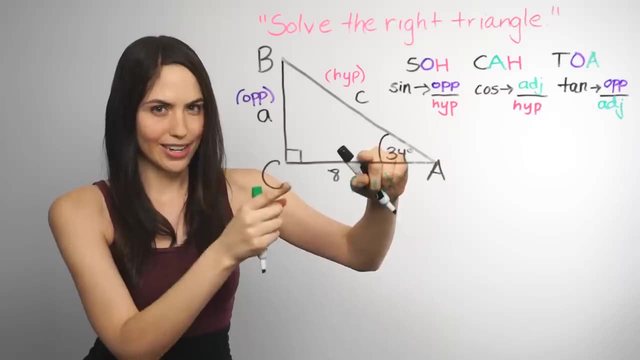 Tangent of 34 degrees, tan 34 degrees equals opposite over adjacent, which for us is A over 8. 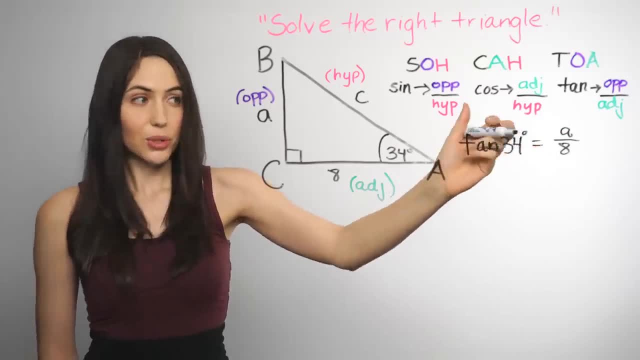 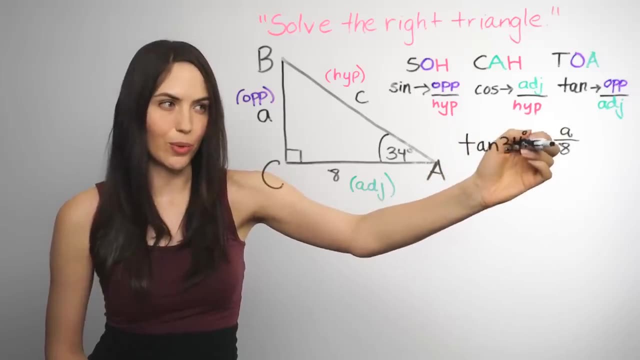 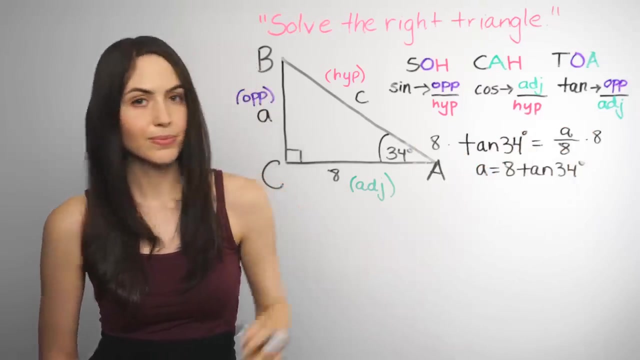 Alright, so here's your equation. You want to solve for A, so you want to get A alone. And right now you have this divided by 8 over there that you don't want. So to undo that or get rid of that, you can multiply by 8. But both sides. Multiply both sides by 8. Okay, so the 8 in the bottom goes away over there and you just have A equals A over A. 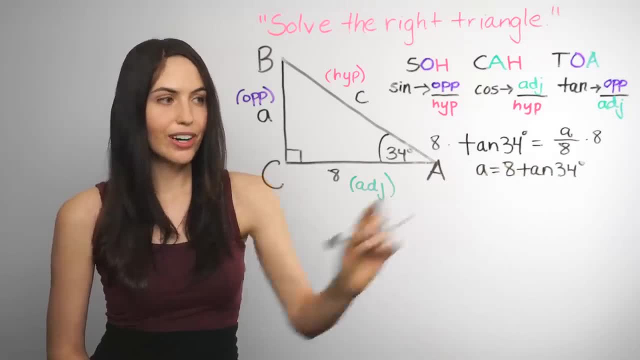 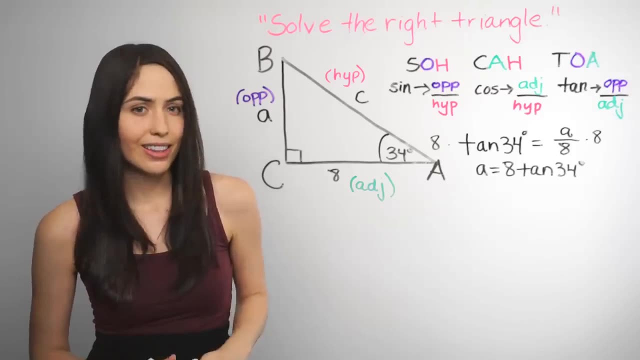 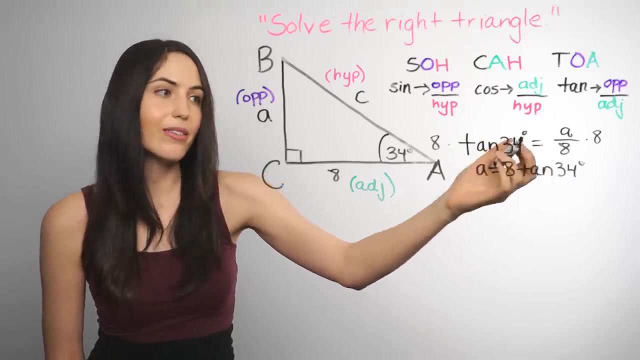 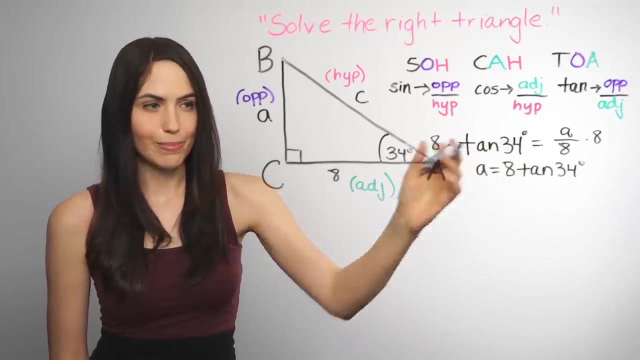 So A equals 8 times tangent 34. A equals 8 times tangent 34. And that's really the answer, but you may have to get an actual number like a decimal and round to the nearest tenth or something like that. So for that you'll need to plug this into your calculator. So either a scientific calculator or a graphing calculator. But make sure that you're in degree mode when you use the tangent 34 degrees and not in radian mode. Otherwise you'll get a weird number that's not right. 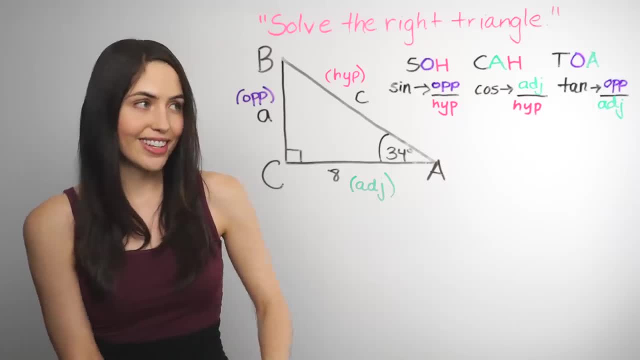 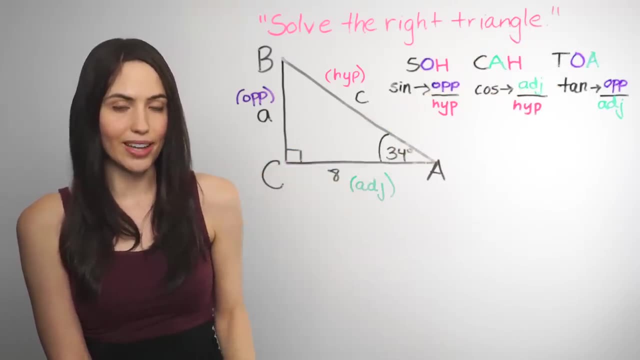 we have 8. Opposite and adjacent, which is the normal side, the one we know for all O and A- you may have already guessed- is tangent trig function. Tan is opposite over adjacent OA, the TOA in SOHCAHTOA. 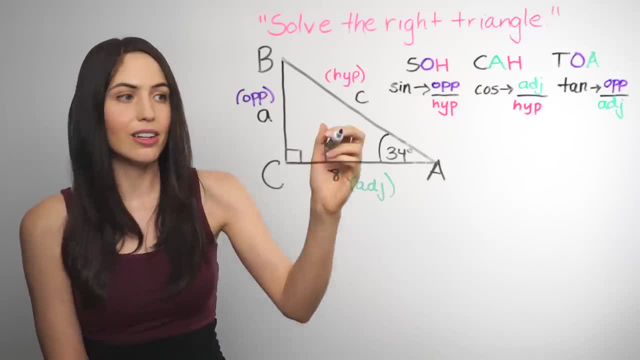 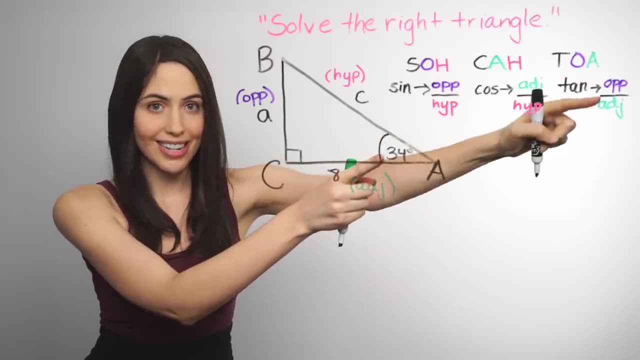 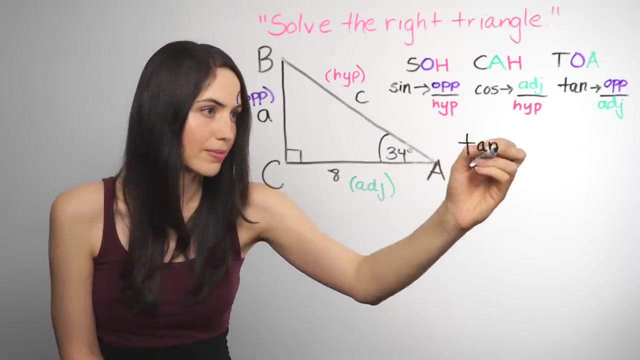 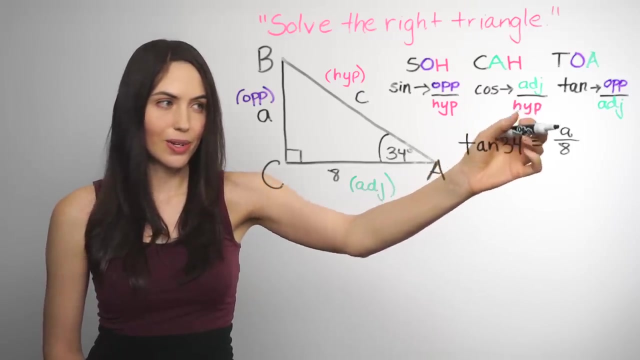 So all we have to do now is write a little equation: tangent of 34 degrees, tan. 34 degrees equals opposite over adjacent, which for us is A over 8.. All right, so here's your equation. You want to solve for A, so you want to get A alone. 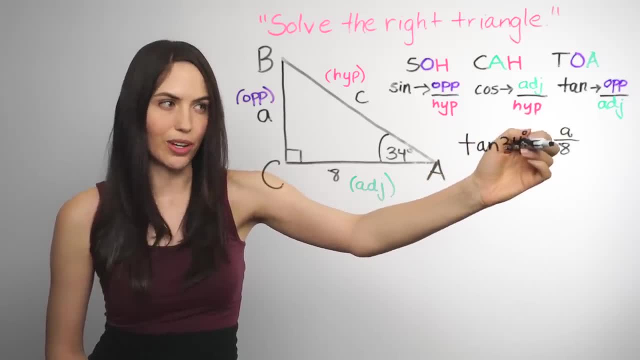 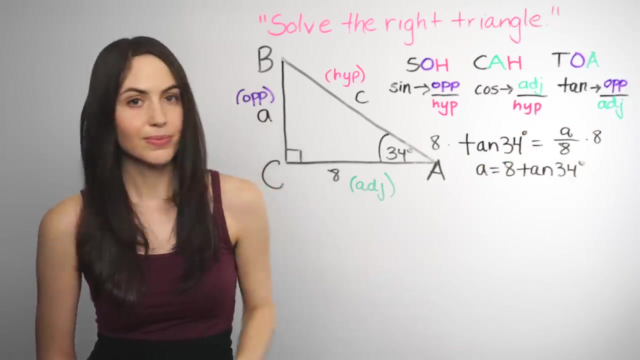 and right now you have this divided by 8 over there that you don't want. So to undo that or get rid of that, you can multiply by 8, but both sides multiply both sides by 8.. Okay, so the 8 in the bottom goes away over there. 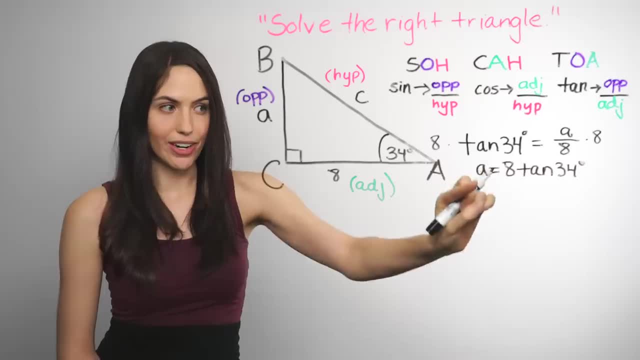 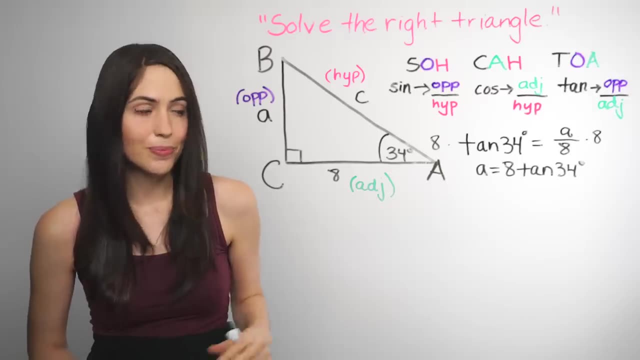 and you just have A equals A. So A equals 8 times tangent 34.. A equals 8 times tangent 34. And that's really the answer. but you may have to get an actual number, like a decimal and round to the nearest tenth or something like that. 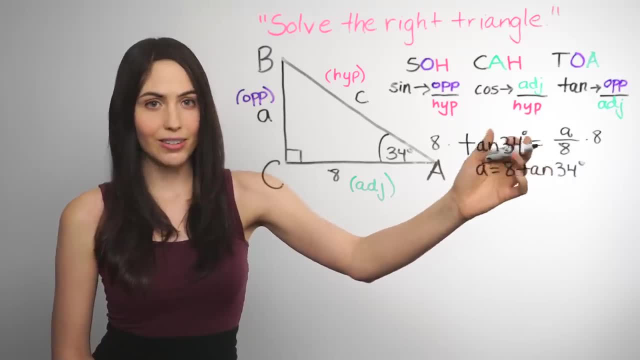 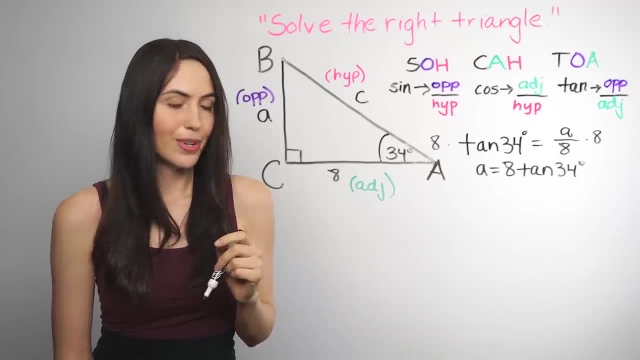 So for that you'll need to plug this into your calculator. so either a scientific calculator or a graphing calculator. but make sure that you're in degree mode when you use the tangent 34 degrees and not in radian mode, Otherwise you'll get a weird number that's not right. 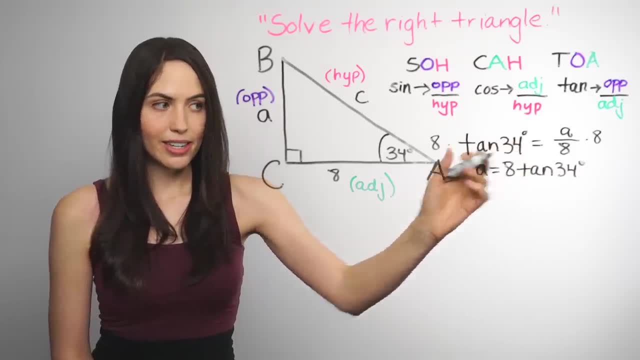 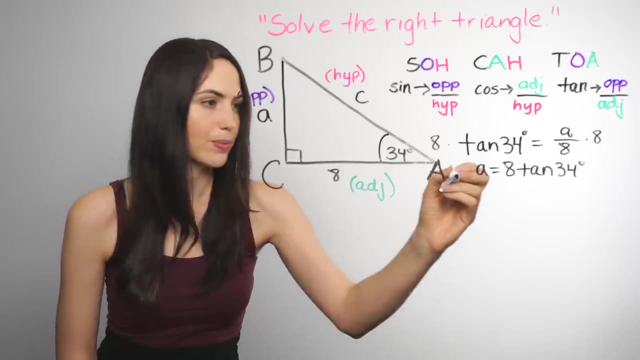 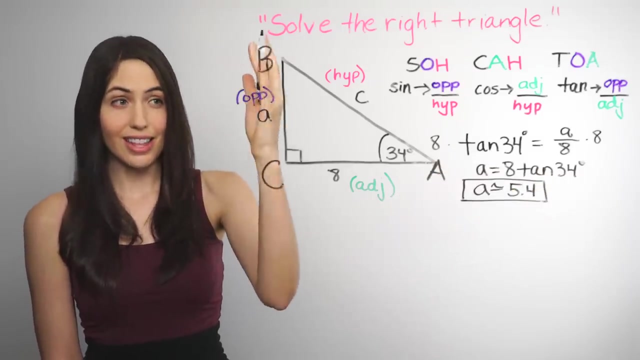 But in degree mode, when you plug in 8 tangent 34 degrees and if you round to the nearest tenth, A is approximately roughly 5.4.. So A is about 5.4.. That opposite side is about 5.4 long. 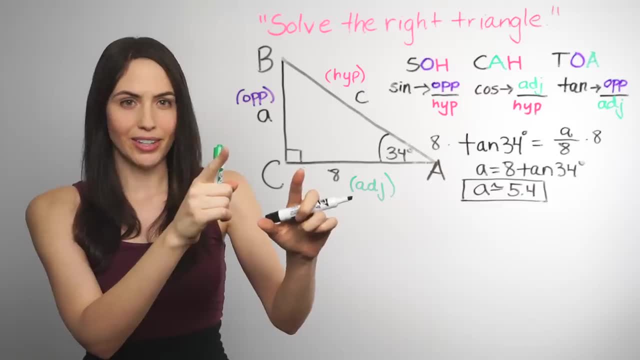 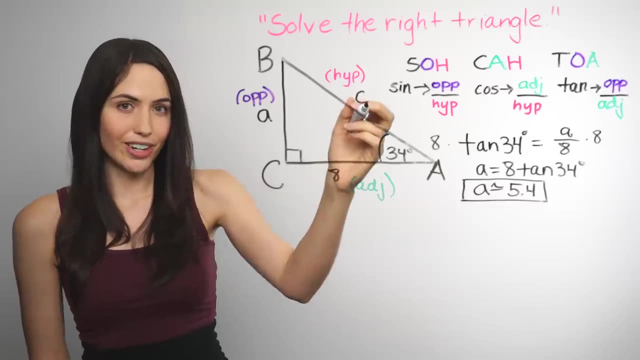 Okay, so you have two sides of the triangle and you don't have the third. There's one side left that you haven't solved for. If you have two sides and you want the third, you have a choice in how you find it. 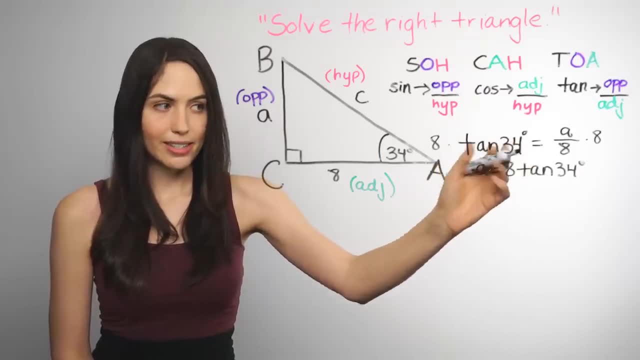 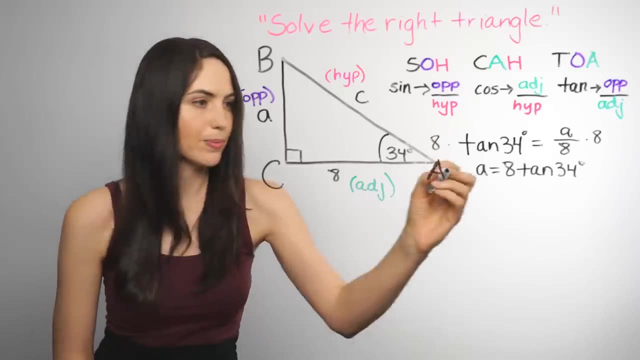 So in degree mode. In degree mode, when you plug in 8 tangent 34 degrees, and if you round to the nearest tenth, it's A is approximately roughly 5.4. So A is about 5.4. That opposite side is about 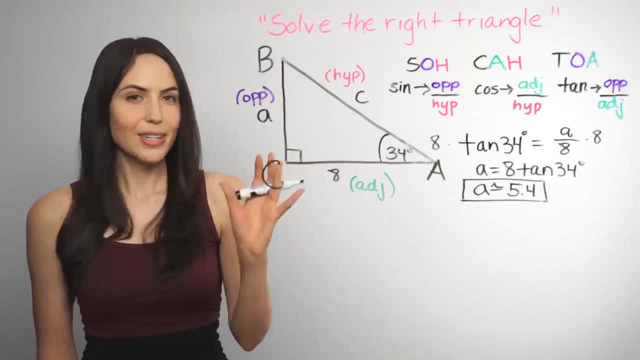 5.4 long. Okay, so you have two sides of the triangle and you don't have the third. There's one side left that you haven't solved for. 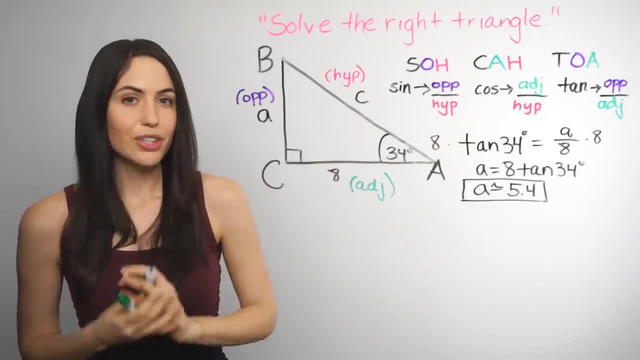 If you have two sides and you want the third, you have a choice in how you find it. You can either use a trig function or you can use Pythagorean theorem. So you can pick your 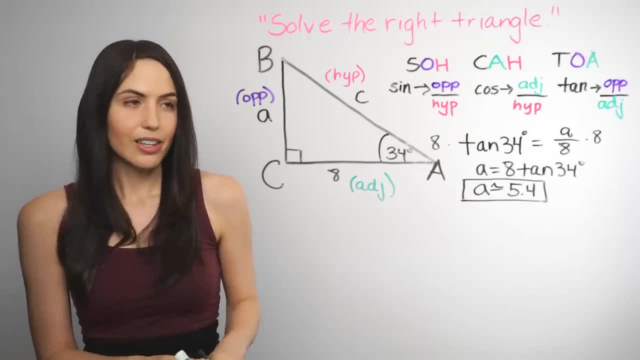 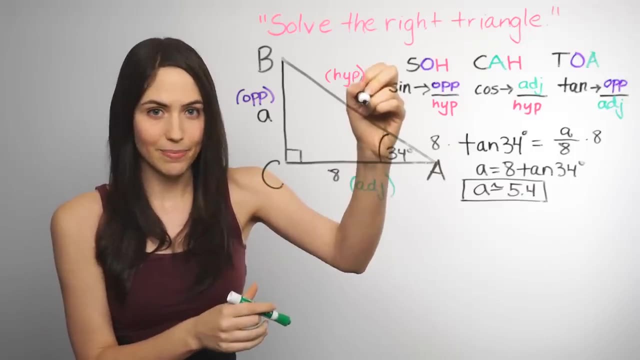 poison, whichever one you want. I'm going to show you both using the trig function. It's the same idea as before. If you want to find this side C, pick the trig function 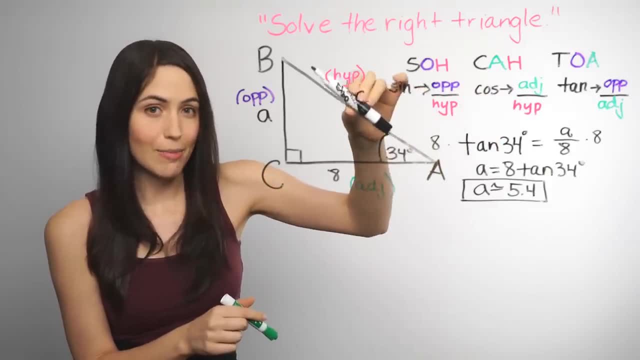 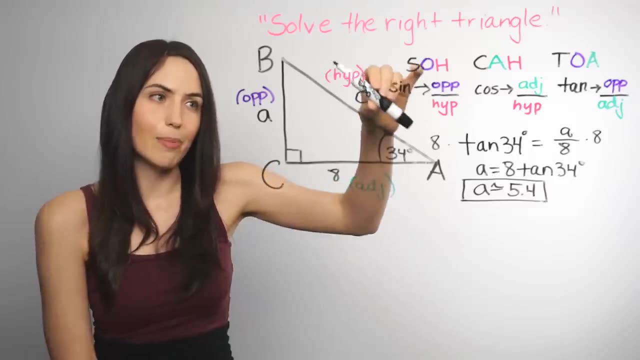 that includes both that side, which is the hypotenuse, and the side that you do know the number for, the value of, which is adjacent. So you want the one that includes hypotenuse 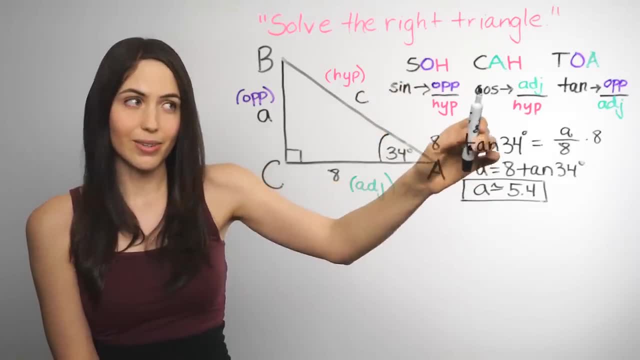 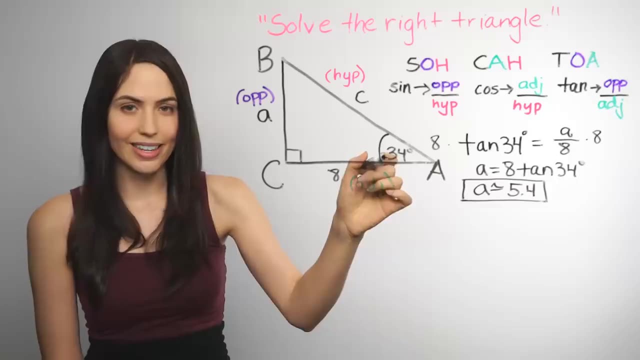 and adjacent, which is cosine, because cosine is adjacent over hypotenuse. So now you just need to write an equation like you did before that's cosine 34 degrees equals adjacent over 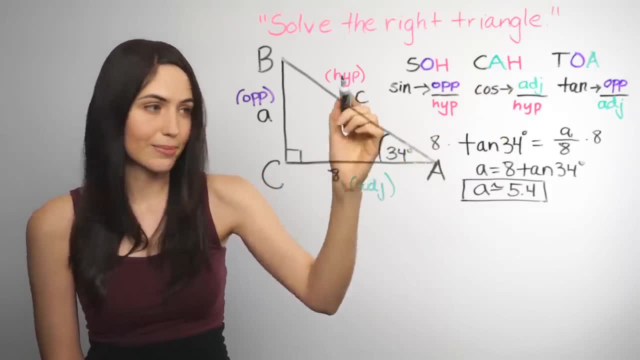 hypotenuse, which is 8 over C. 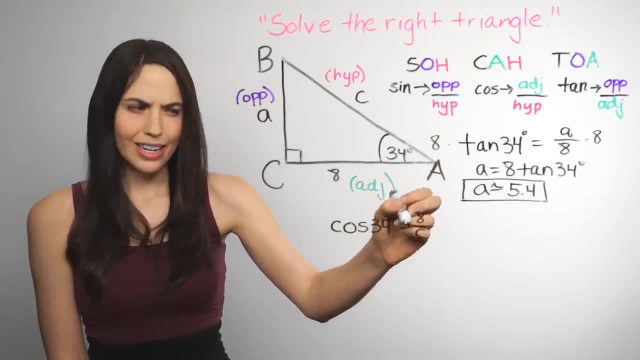 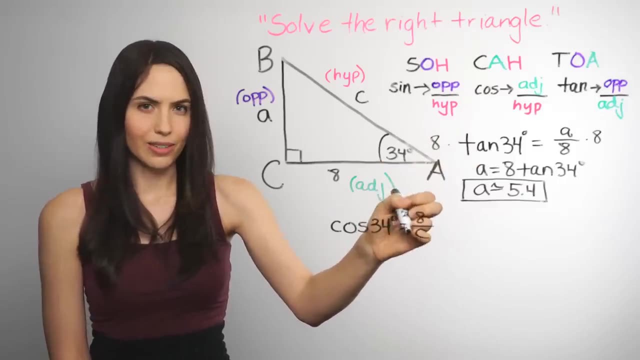 Okay, and you want to solve for C. It's down there in the denominator in the bottom, which is different from the one before. How do you solve when the variable you want is down in 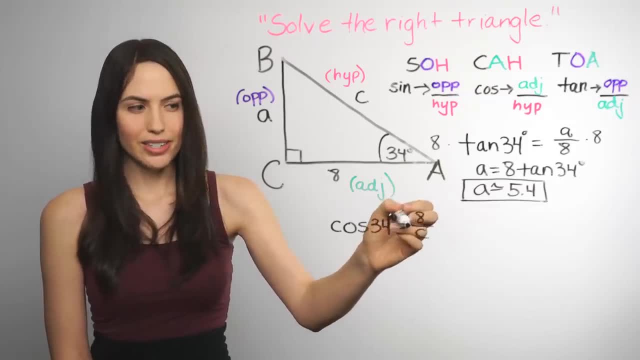 the denominator? There's an extra step. You want to get rid of it in the denominator and bring it up top, and the trick is multiply both sides by C so that you clear it over there and bring it up on one side. So multiply both sides by C. 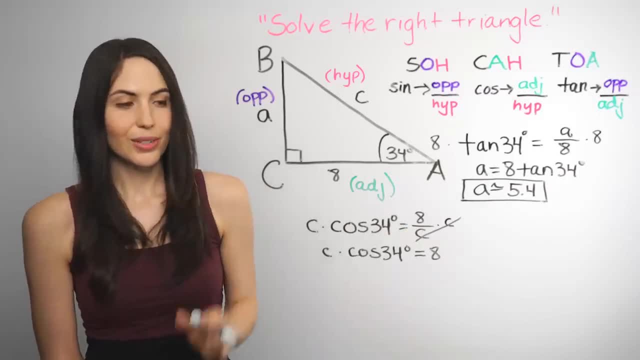 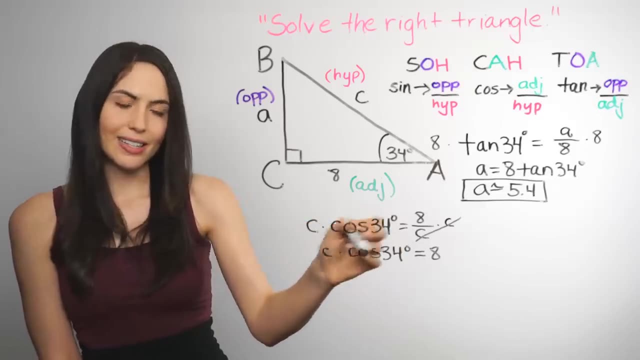 So we're closer. You have C here, but you also have this times cosine 34 degrees. You want to get C alone, so anything that's attached that you don't want there, divide out. So 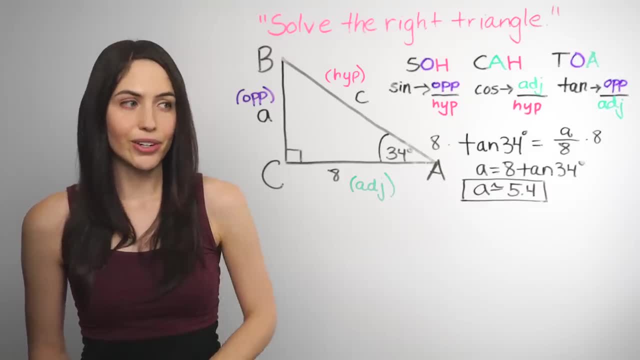 You can either use a trig function or you can use Pythagorean theorem, So you can pick your poison, whichever one you want. I'm going to show you both using the trig function. It's the same idea as before, If you want to find this side C. 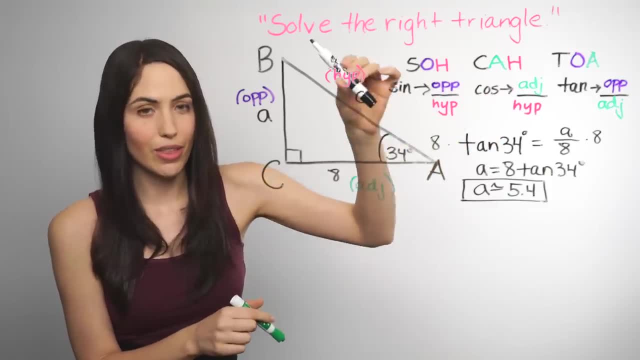 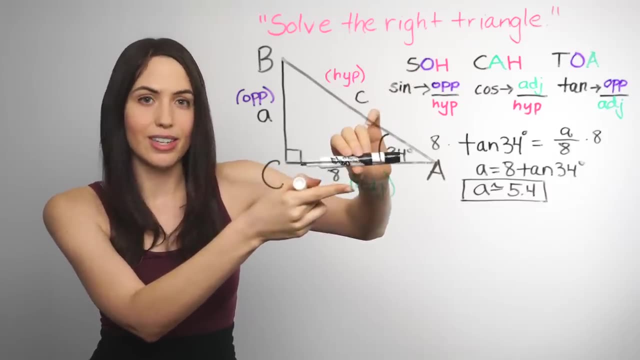 pick the trig function that includes both that side, which is the hypotenuse, and the side that you do know, the number for the value of which is adjacent. So you want the one that includes hypotenuse and adjacent, which is cosine. 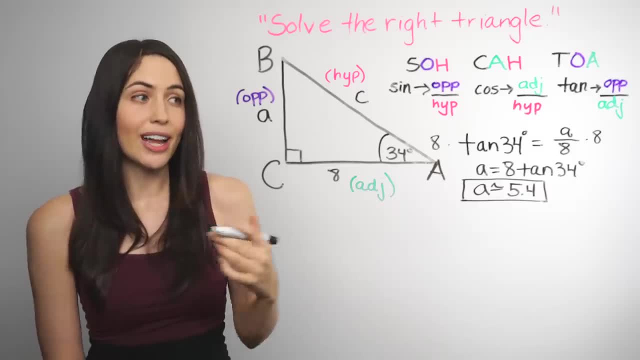 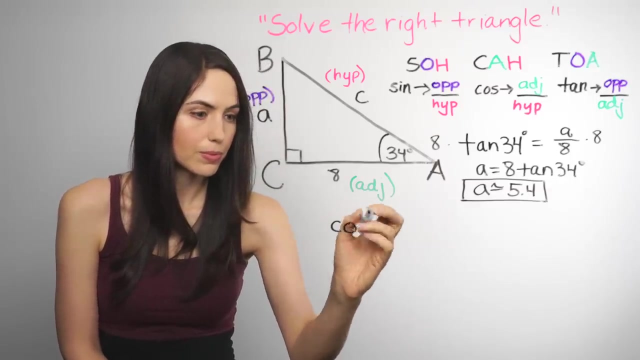 because cosine is adjacent over hypotenuse. So now you just need to write an equation, like you did before. that's: cosine, 34 degrees equals adjacent over hypotenuse, which is 8 over C. Okay, and you want to solve for C? 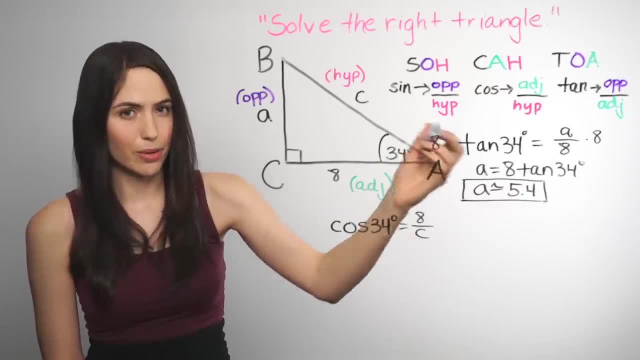 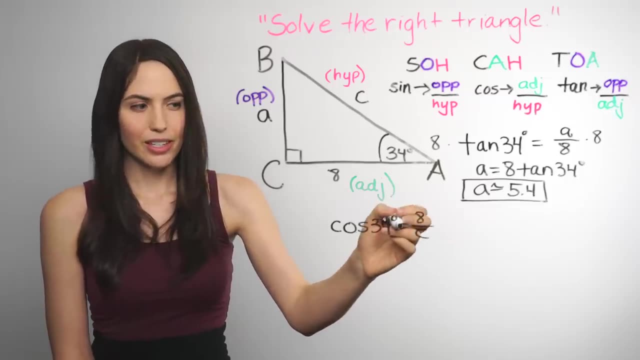 It's down there in the denominator, in the bottom, which is different from the one before. How do you solve when the variable you want is down in the denominator? There's an extra step. You want to get rid of it in the denominator and bring it up top. 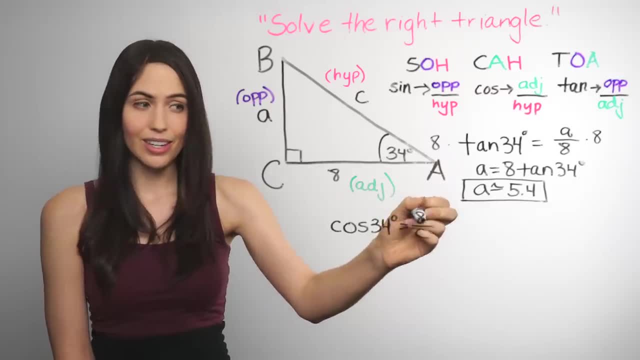 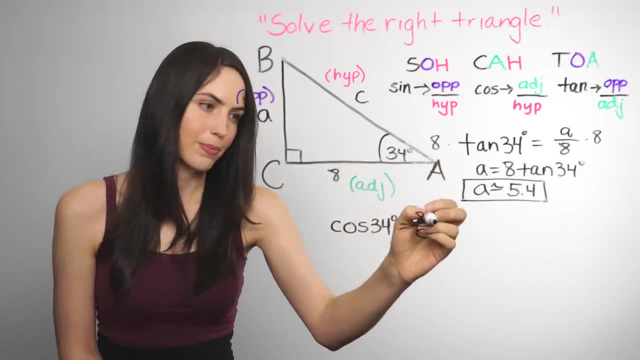 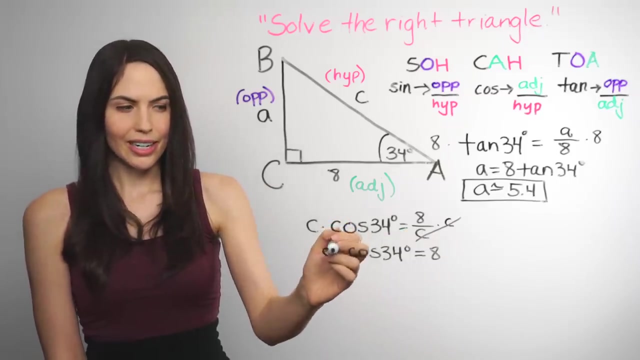 and the trick is: multiply both sides by C so that you clear it over there and bring it up on one side. Multiply both sides by C So you're closer. You have C here, but you also have this times cosine 34 degrees. 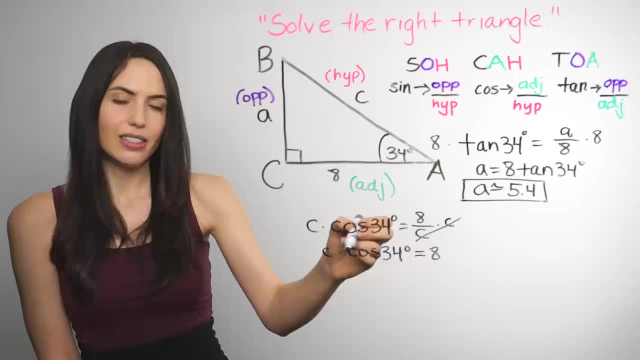 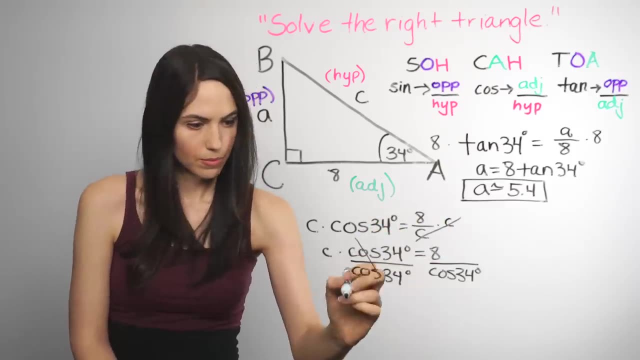 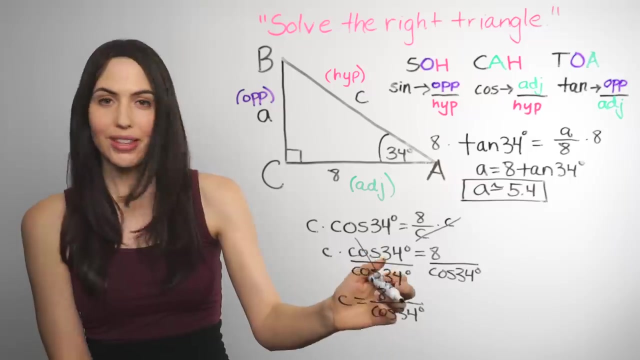 You want to get C alone. so anything that's attached that you don't want there divide out. So divide both sides by cosine 34 degrees. So C is equal to 8 divided by cosine 34 degrees. Again, just put this in your calculator. 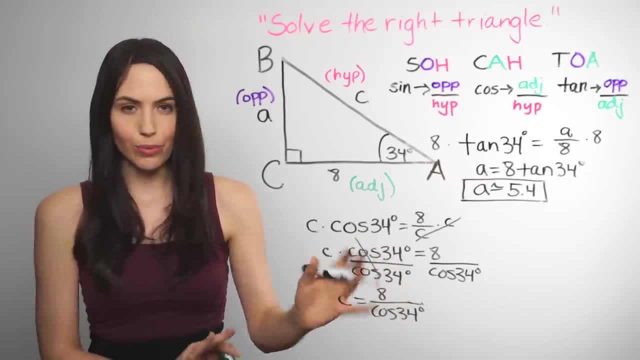 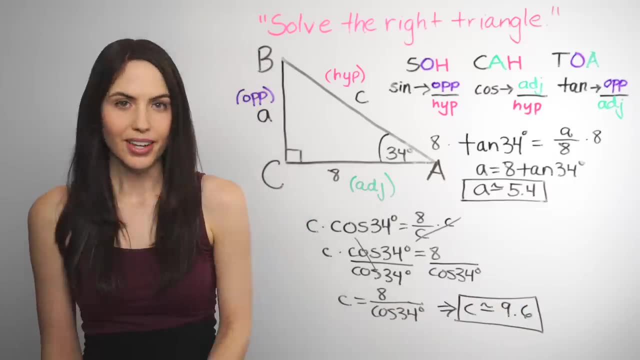 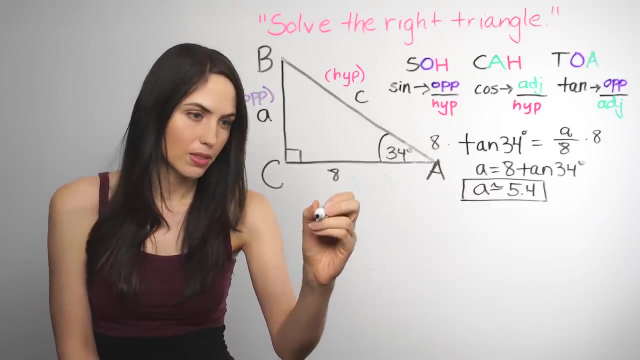 Using degree mode and if you round it it's roughly 9.6.. Okay, so there's another way to find that last side. Like I said, you could use the Pythagorean theorem. Okay, so here's the Pythagorean theorem. 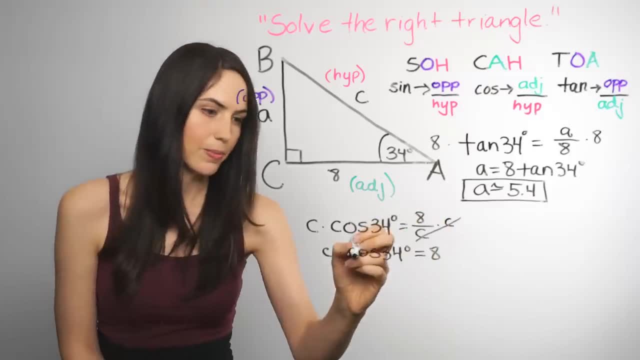 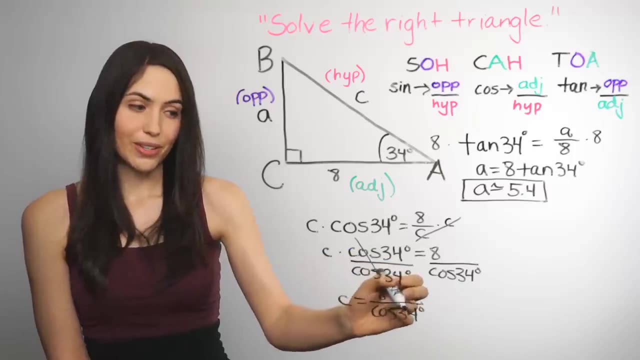 divide both sides by cosine 34 degrees. So C is equal to 8 divided by cosine 34 degrees. Again, just put this in your calculator using degree mode, and if you round it, it's going to be the same. 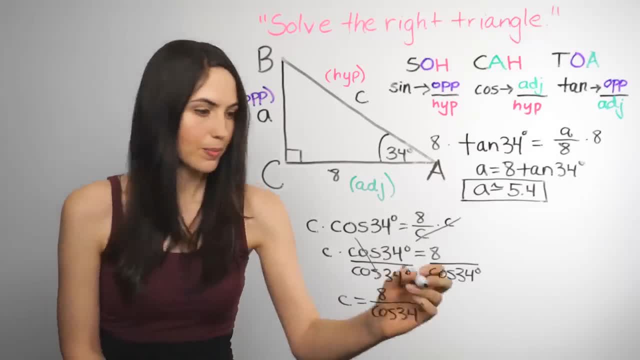 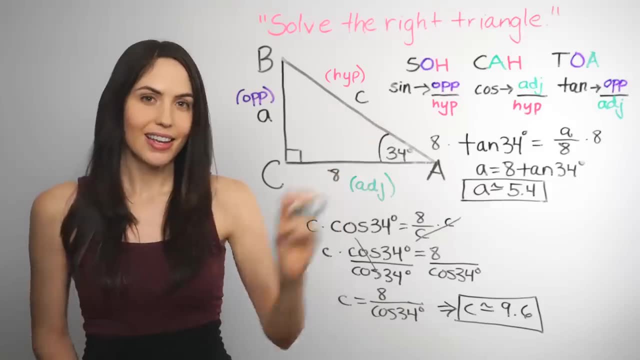 And it's roughly 9.6. Okay, so there's another way to find that last side. Like I said, you could use the 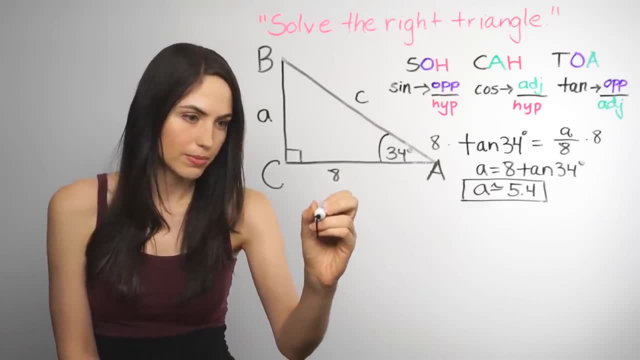 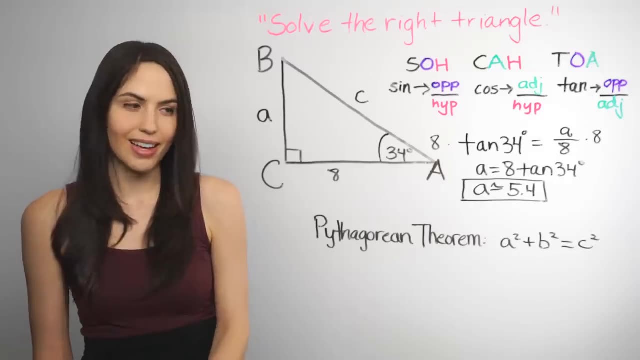 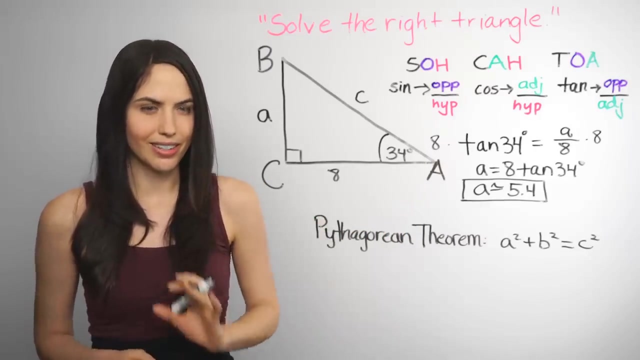 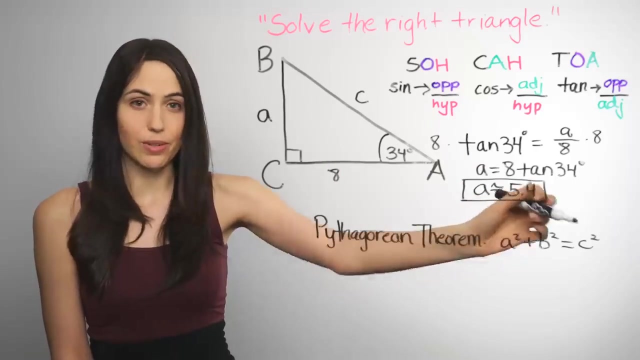 Pythagorean theorem. Okay, so here's the Pythagorean theorem, or Pythag as the cool kids say. Just don't call it the Pythagorean theorem like I did when I was little. It's definitely wrong. Definitely wrong. weird and the wrong emphasis for the syllables. But basically, it's a squared plus b squared equals c squared, and hopefully you've seen it before. C is always the hypotenuse, and 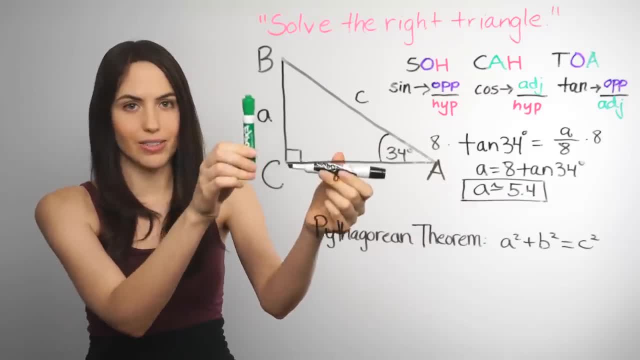 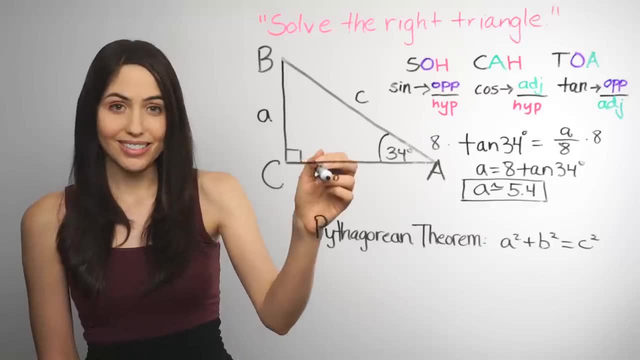 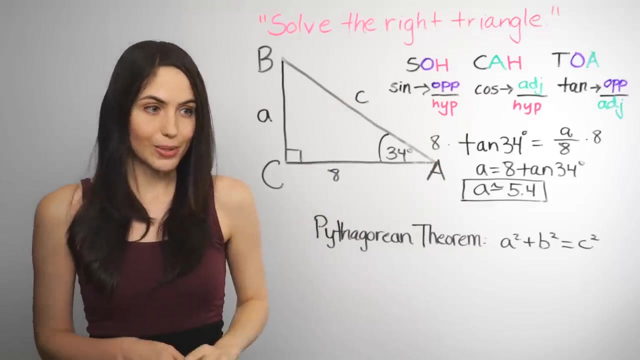 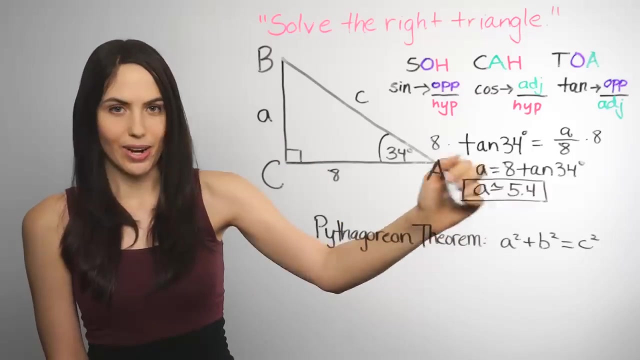 a and b are the legs of the triangle that are on either side of the right angle. If you have two of them, you can find the other. And we have b. We did find a earlier with our tangent. It was about 5.4. And we want c, so we can use the numbers that we have for a and b and plug them in and solve for c. And it's better to use the unrounded decimal, 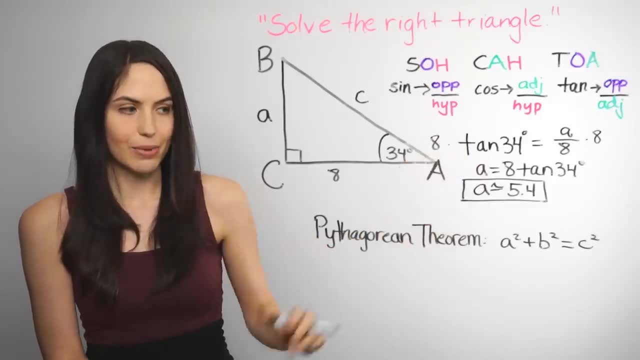 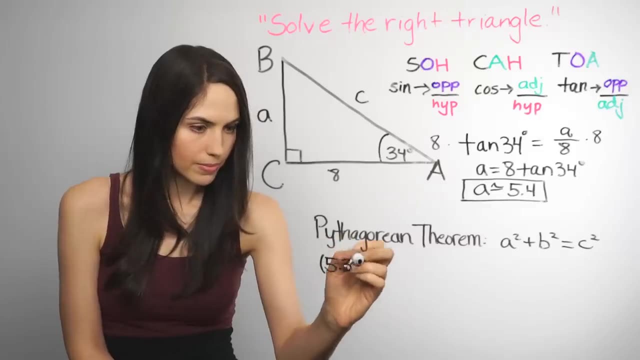 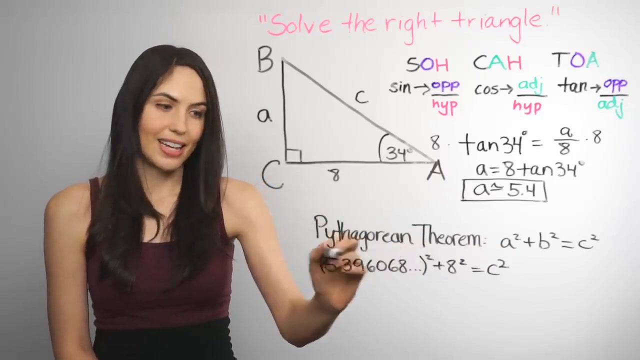 by the way, which hopefully you still have in your calculator, because that will give you a more accurate answer in the end. So when you plug it in, it looks like this. And And this, if you square it, turns out to be 29 point something plus 8 squared, 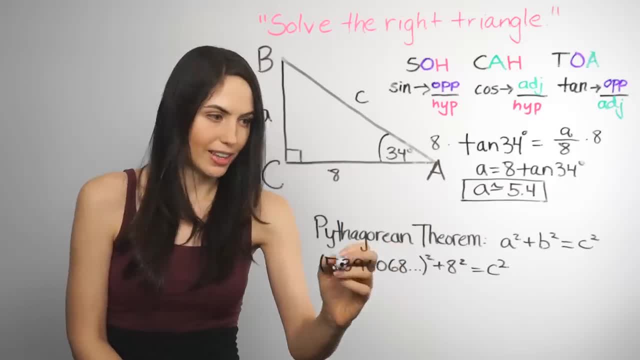 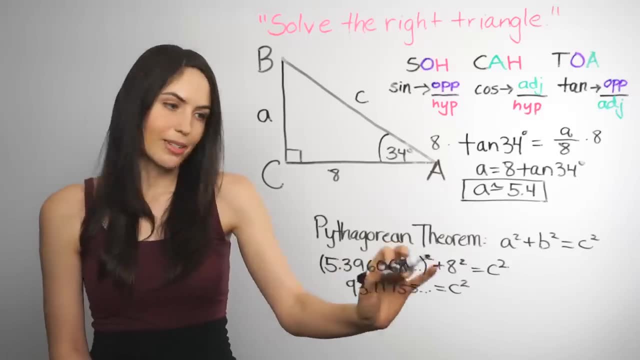 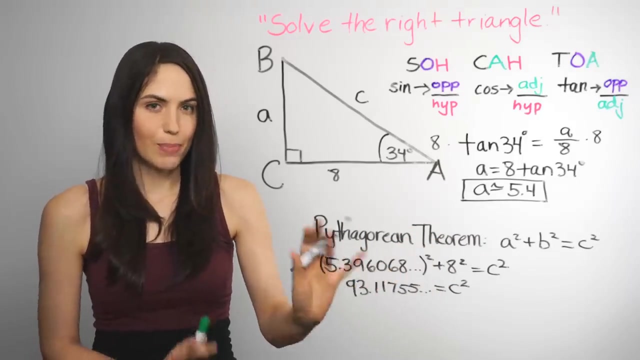 which is 64, so all together it would look like this. So it's 93 point something something something equals c squared, and to get just c, you can square root both sides to get c alone, and use the positive answers, since this is a length, 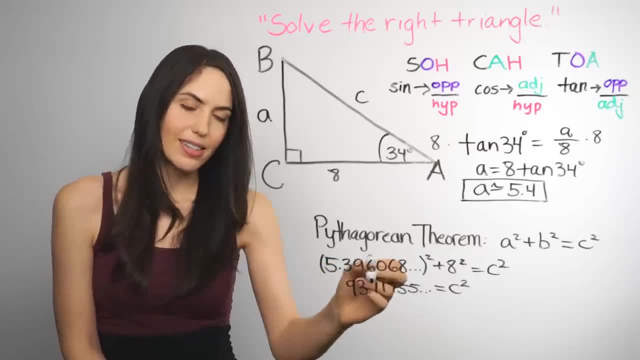 a distance that should be positive, and when you do that, c is about 9 point 6, which we knew already. 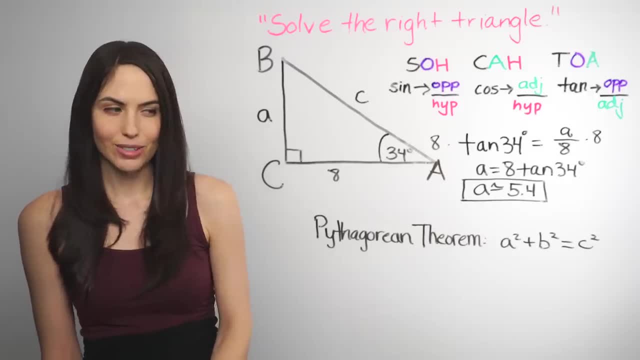 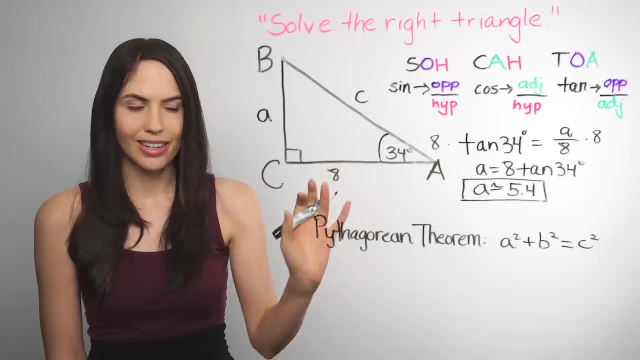 or Pythag as the cool kids say. Just don't call it the Pythagorean theorem, Like I did when I was little. It's definitely wrong, Definitely weird, and the wrong emphasis for the syllables, But basically it's A squared plus B squared equals C squared. 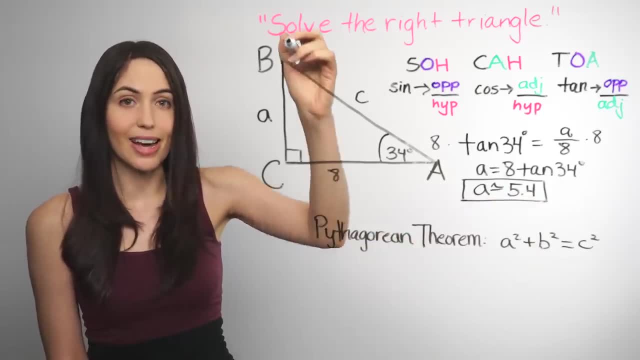 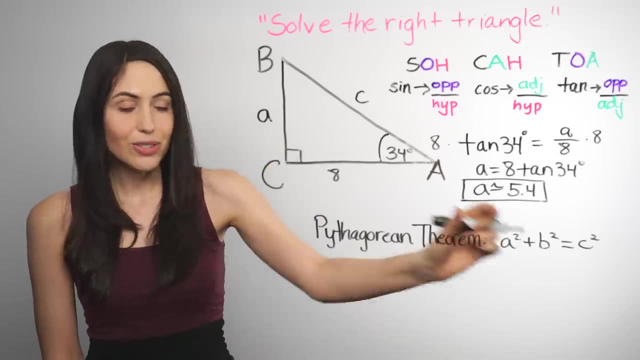 and hopefully you've seen it before. C is always the hypotenuse and A and B are the legs of the triangle that are on either side of the right angle. If you have two of them, you can find the other, And we have B. 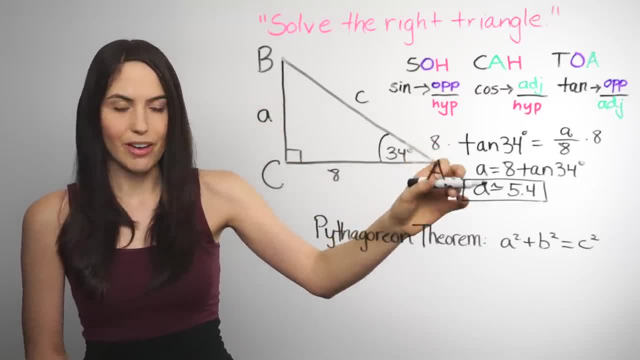 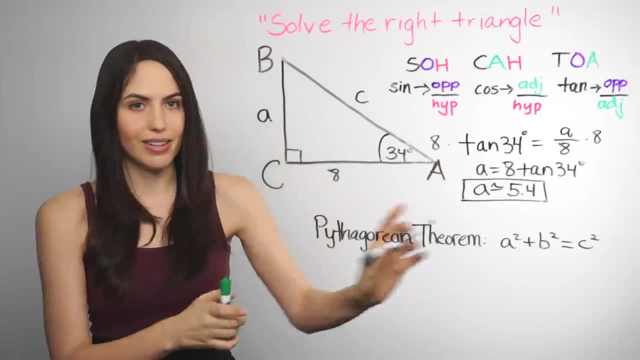 We did find A earlier with our tangent- It was about 5.4, and we want C. So we can use the numbers that we found, for we have for A and B and plug them in and solve for C, And it's better to use the unrounded decimal. 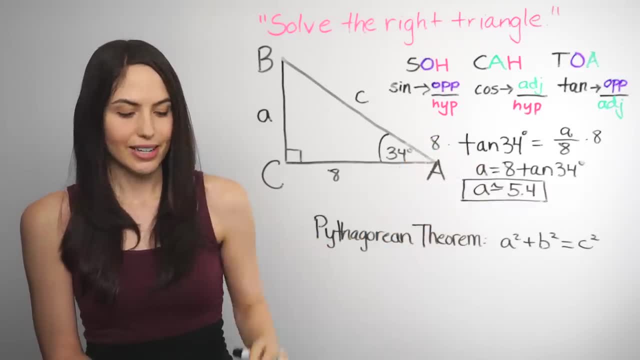 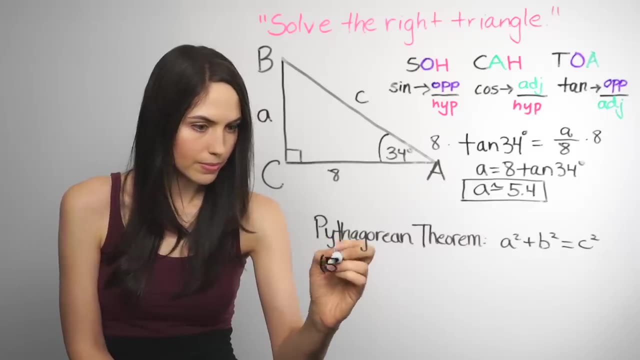 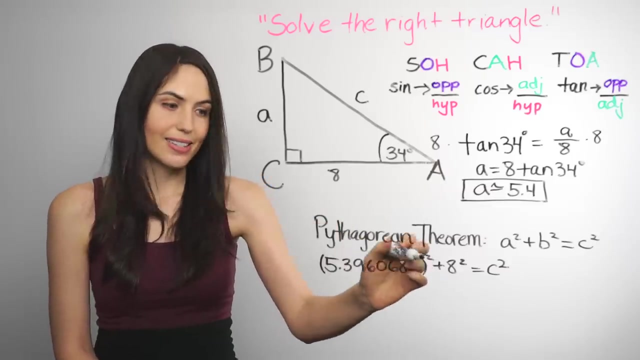 by the way, which hopefully you still have in your calculator, because that will give you a more accurate answer in the end. So when you plug it in, it looks like this And this: if you square it turns out to be 29 point something plus 8 squared. 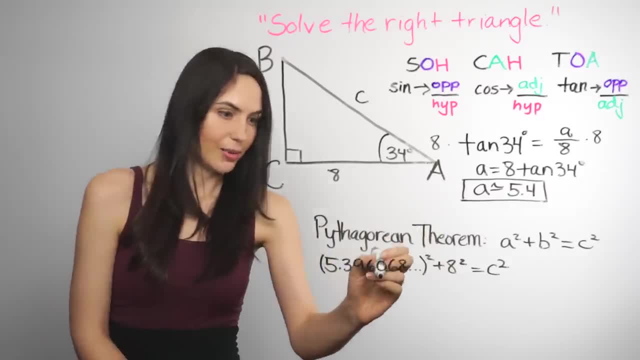 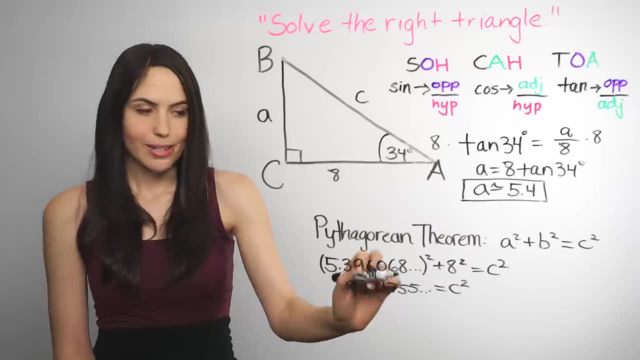 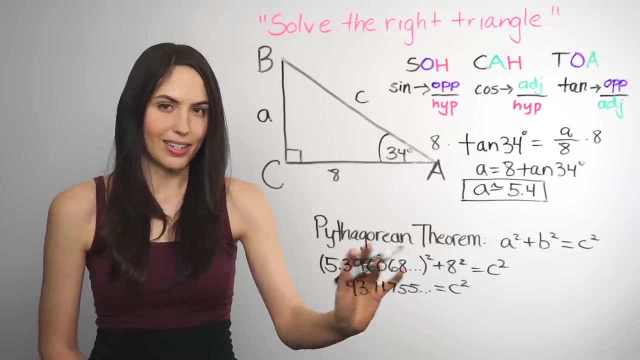 which is 64.. So altogether it would look like this: So it's 93 point something, something. something equals C squared, and to get just C, you can square root both sides to get C alone and use the positive answers, since this is a length. 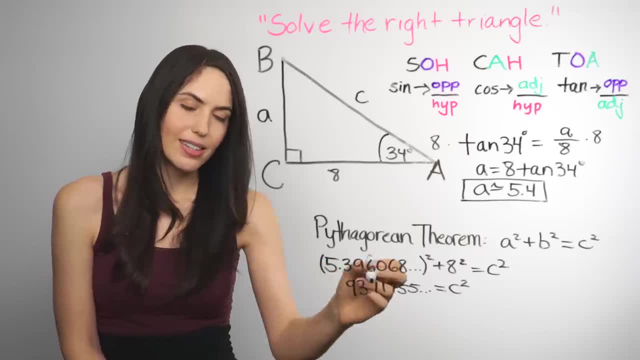 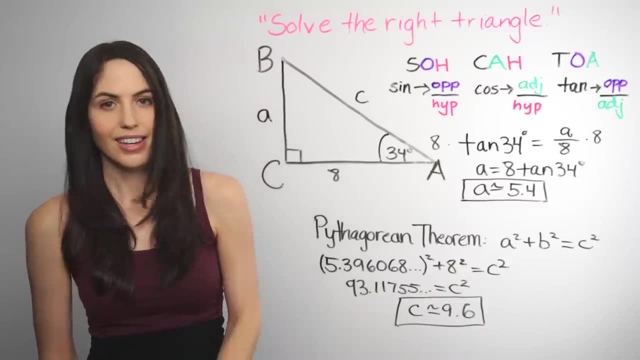 a distance that should be positive, And when you do that, C is about 9.6, which we knew already. So that's how you can use the Pythagorean Theorem, and we found that the hypotenuse is about 9.6 long. 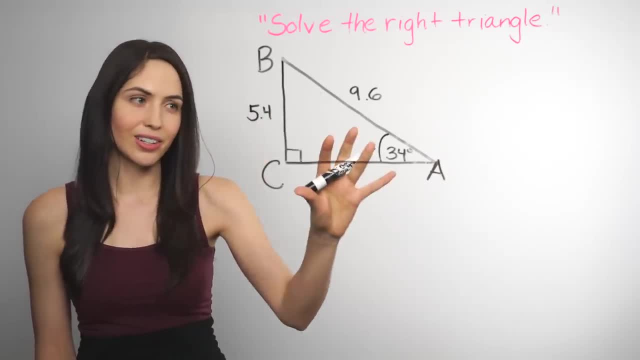 Okay, so you've found all the sides of the triangle and I know you may think you're done, but there's one last thing to figure out and clearly label, and it's this other angle, because it's not already clearly labeled. 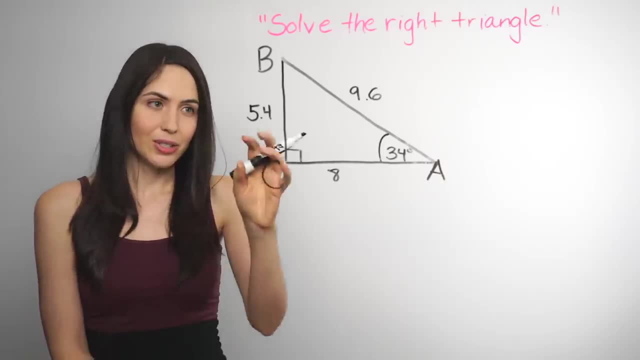 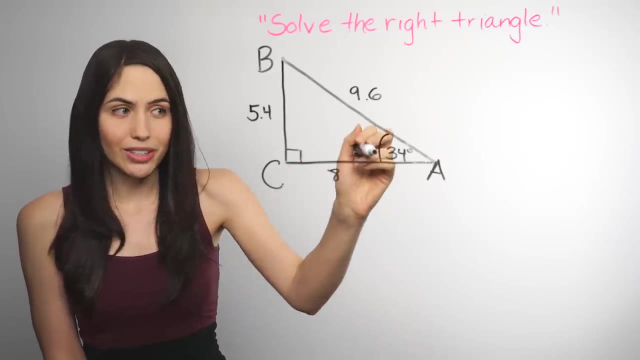 Don't worry, this is the fastest, easiest part, because in a triangle all the angles inside have to add up to 180 degrees. So if we we know for sure that this is 34 degrees and this angle here is 90 degrees, 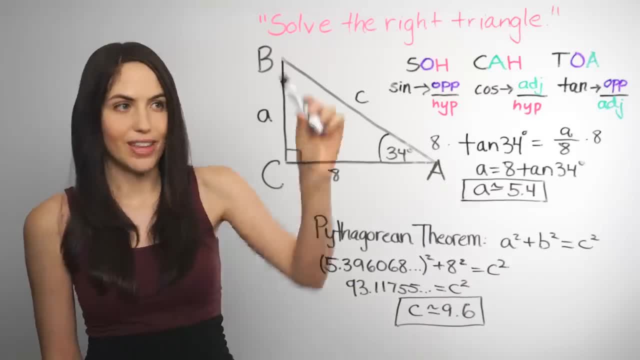 So that's how you can use the Pythagorean Theorem, and we found that the hypotenuse is about 9 point 6 long. 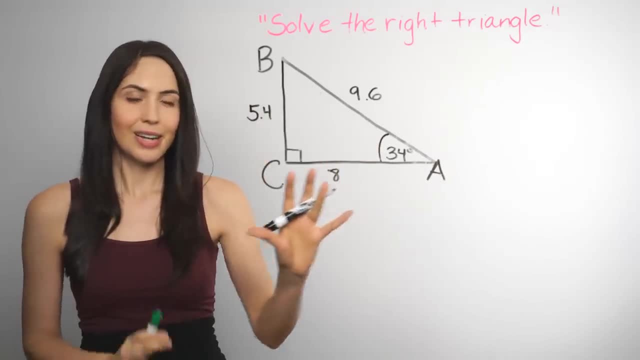 Okay, so you've found all the sides of the triangle, and I know you may think you're done, but there's one last thing to figure out and clearly label, and it's this other angle. 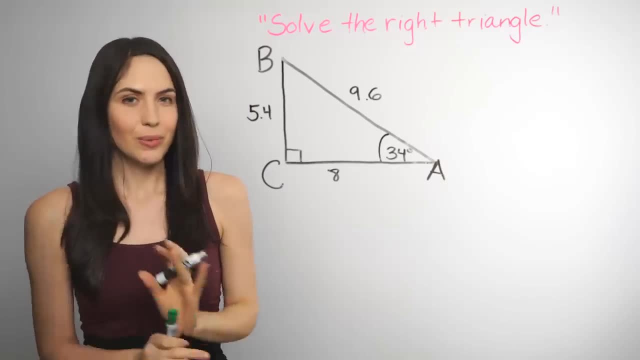 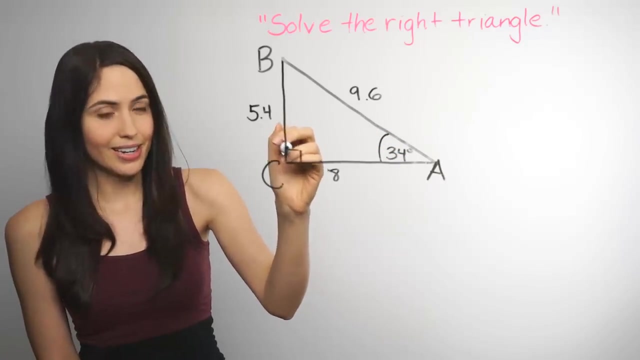 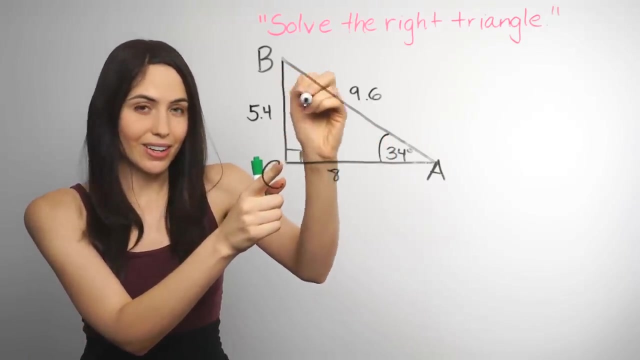 It's not already clearly labeled. Don't worry, this is the fastest, easiest part, because in a triangle, all the angles inside have to add up to 180 degrees, so if we know for sure that this is 34 degrees, and this angle here is 90 degrees, because it's a right angle, we know that the 90 and 34 and whatever this other angle is better equal 180 degrees, and we can write an equation that says that. 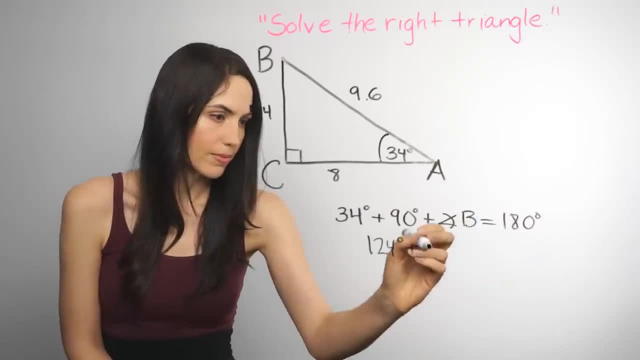 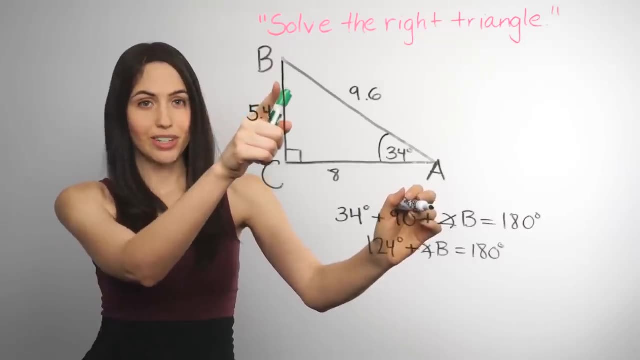 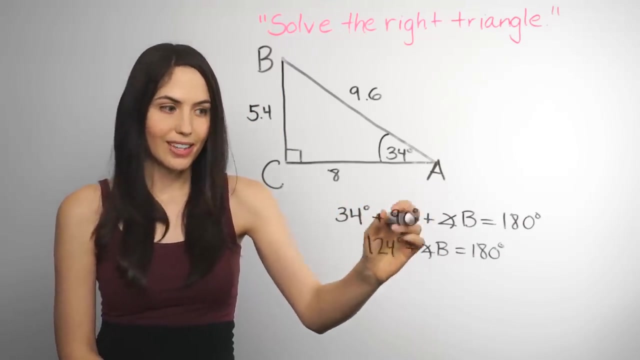 So here's the equation. All three angles, including angle B, which we're looking for, have to equal 180. If we clean this up, those two together are 124, and if you subtract that from both sides, you'll see that angle B has to be 56 degrees. 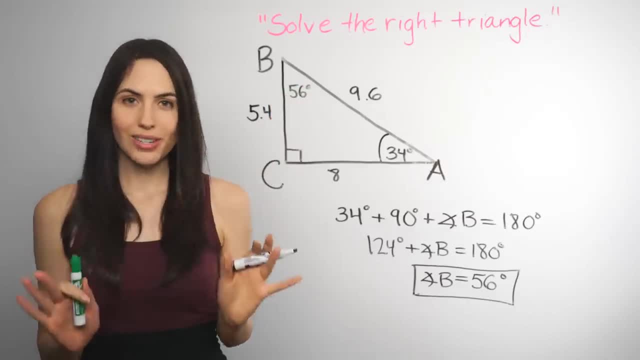 So that angle is 56 degrees, and the triangle is totally solved. All sides and angles are labeled, and you're done. 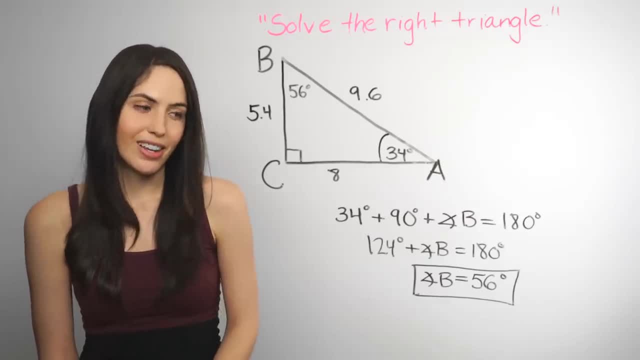 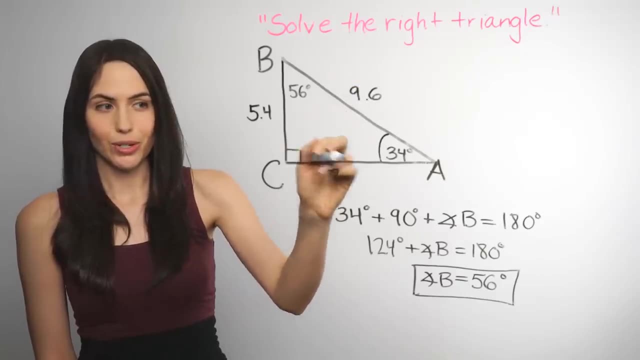 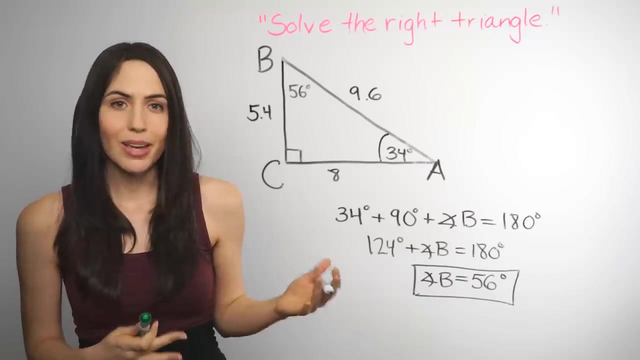 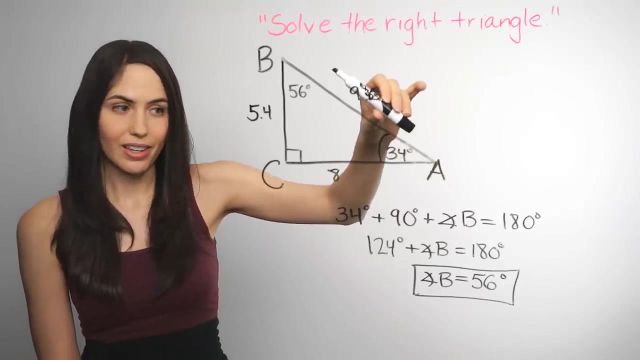 Just a few things I want to mention. If you got a different side given to you in the beginning, like if you weren't told this side, but you were instead given the hypotenuse and no other sides, don't worry. It's the same kind of steps. Just make sure you pick a trig function that includes both that hypotenuse you know and whatever side you're looking for. 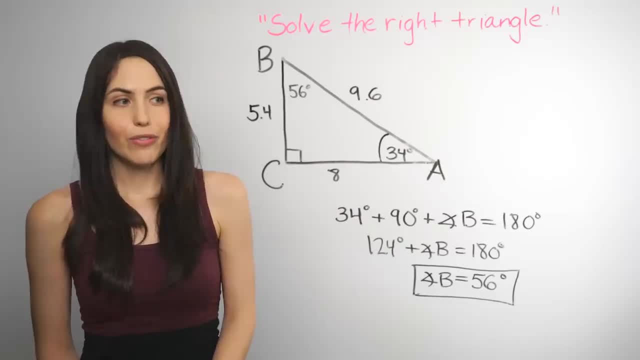 So it's the same idea. Also, if you are given no angles in the beginning, other than the 90-degree angle, 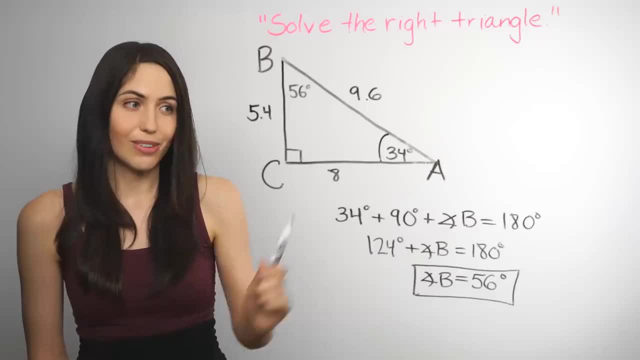 you may need to use inverse trig functions to find an angle and fully solve, and that's a whole other video if you see that. 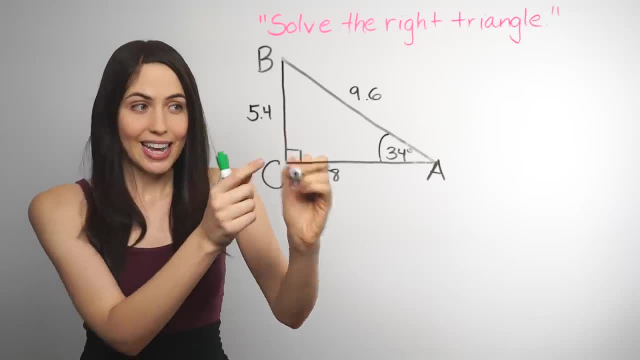 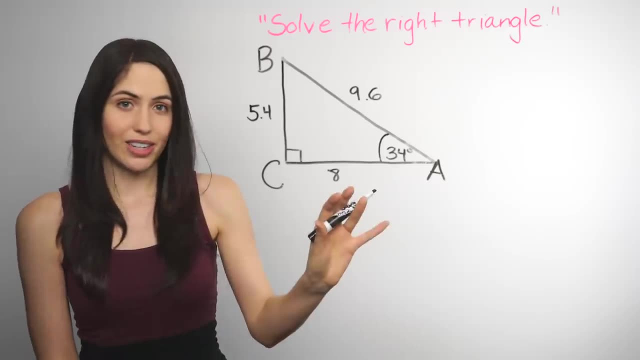 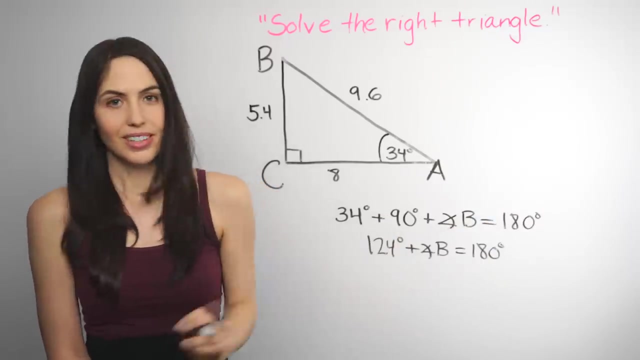 because it's a right angle. we know that the 90 and 34, and whatever this other angle is better- equal 180 degrees, and we can write an equation that says that. So here's the equation: All three angles, including angle B. 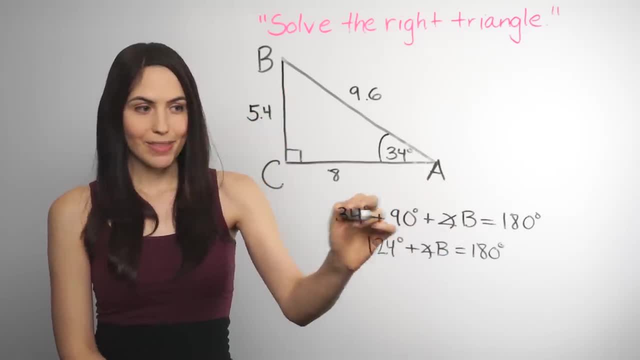 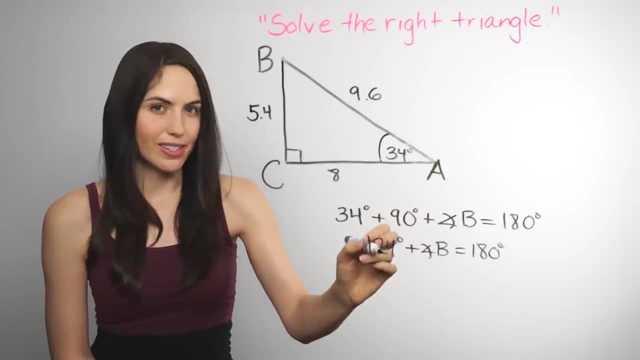 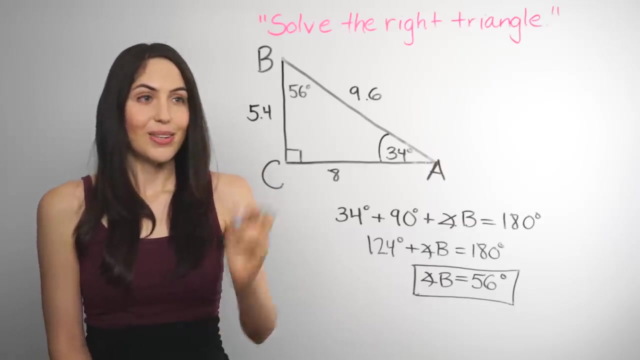 which we're looking for, have to equal 180.. If we clean this up, those two together are 124, and if you subtract that from both sides you'll see that angle B has to be 56 degrees, So that angle is 56 degrees. 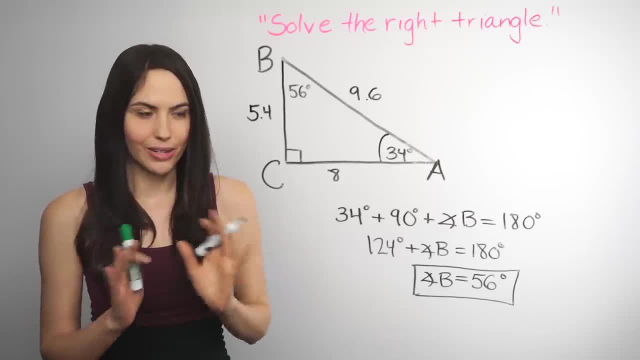 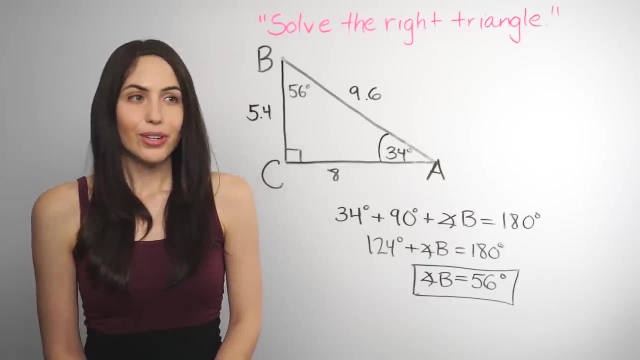 and the triangle is totally solved, All sides and angles are labeled and you're done. Just a few things I want to mention. If you got a different side given to you in the beginning- like if you didn't weren't told this side- 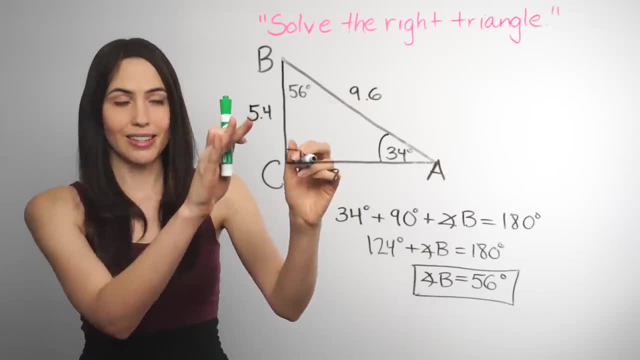 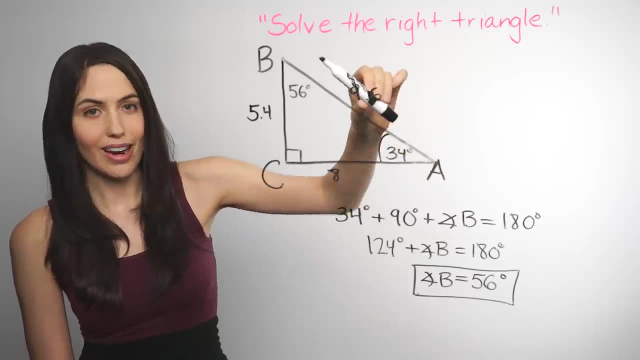 but you were instead given the hypotenuse and no other sides. don't worry, it's the same kind of steps. Just make sure you pick a trig function that includes both that hypotenuse, you know, and whatever side you're looking for. 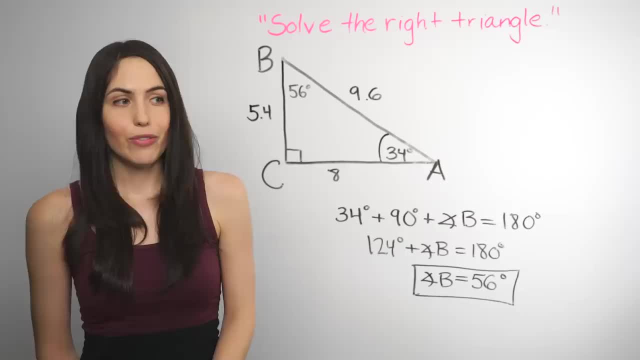 So it's the same idea. Also, if you are given no angles in the beginning other than the 90 degree angle, you may need to use inverse trig functions to find an angle and fully solve. and that's a whole other video. if you see that, 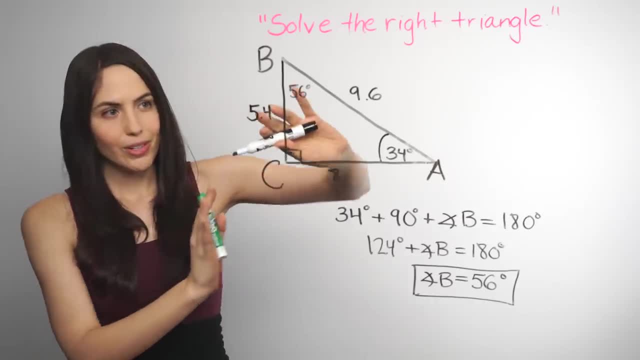 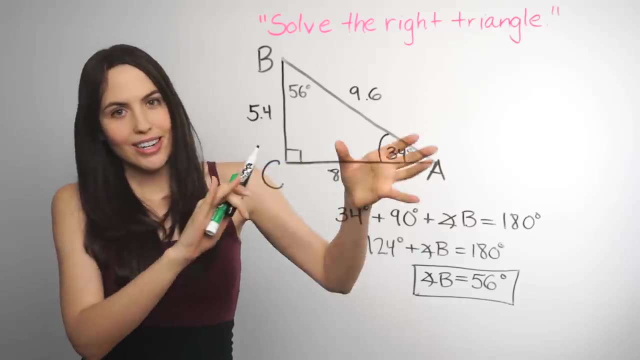 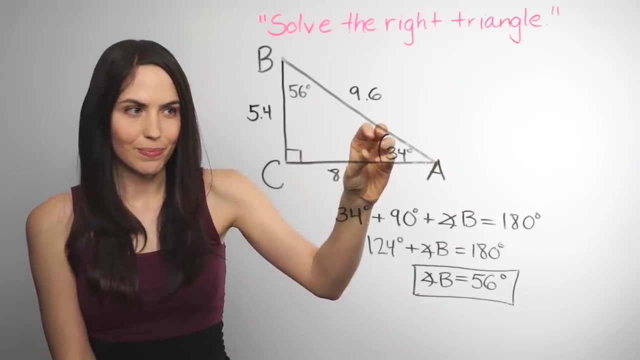 And one last thing: don't worry if you see a triangle given to you that's like rotated, it's oriented differently. No matter what orientation you get, it's the same idea. Just focus on an angle, figure out for yourself which side is opposite. 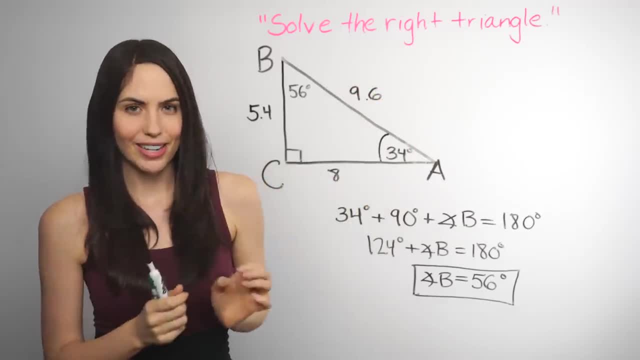 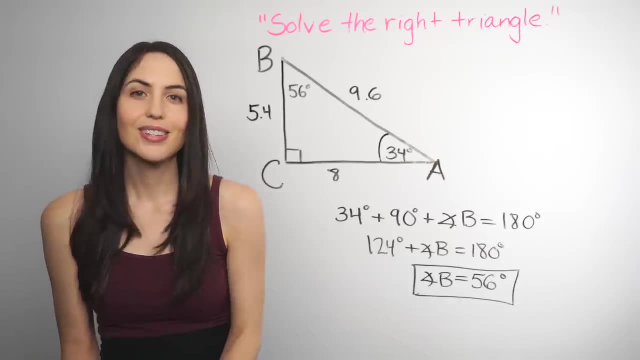 which side is hypotenuse, which side is adjacent to it, and then pick a trig function, knowing what you have and what you need. So it's the same kind of steps. So I hope that helped you understand how to solve right triangles with trig.